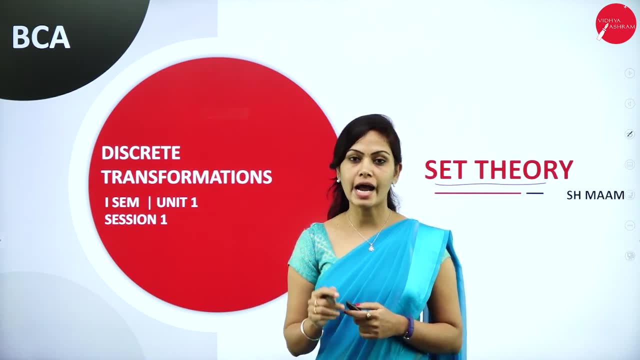 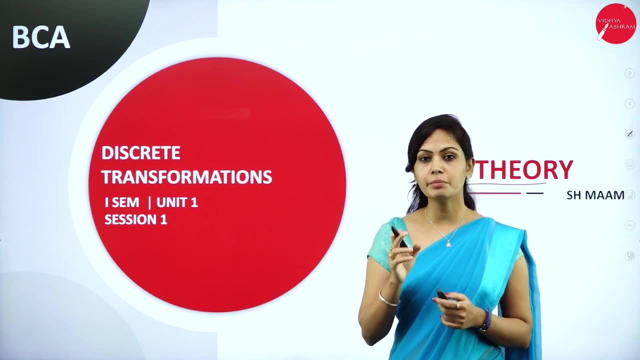 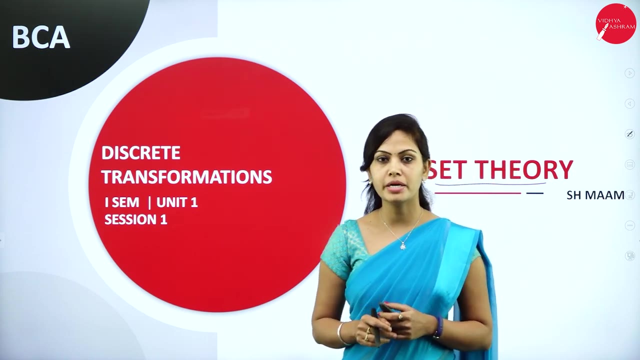 And it is very good tool for improving reasoning and problem solving capabilities. So discrete transformation is a branch of mathematics and it is increasingly being applied in the practical field of computer science and mathematics. So using this discrete mathematics, you can improve your problem solving ability. 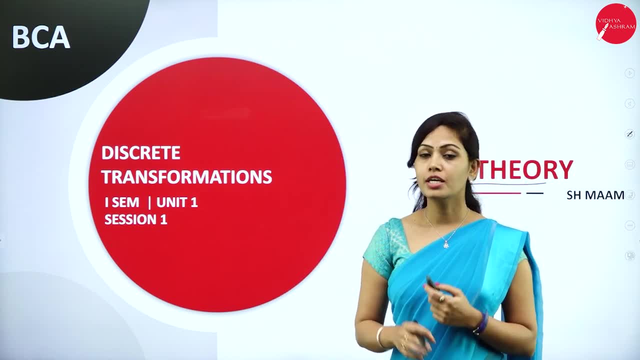 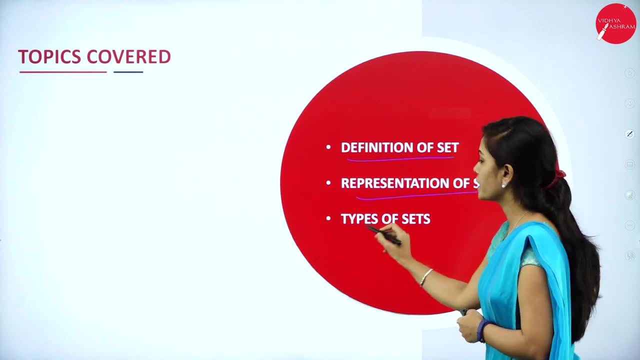 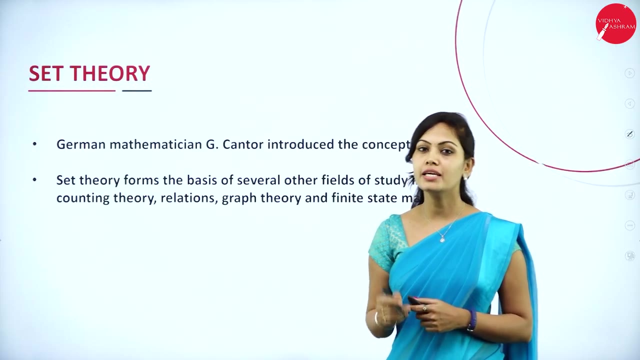 So now I will discuss about set theory. So in my today's session I will discuss The following topics: definition of set, representation of sets and types of sets. So what is set theory? Set theory was introduced by German mathematician G Cantor. introduced of the concepts of sets. 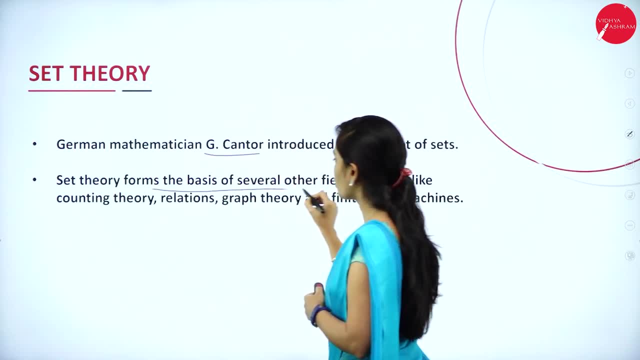 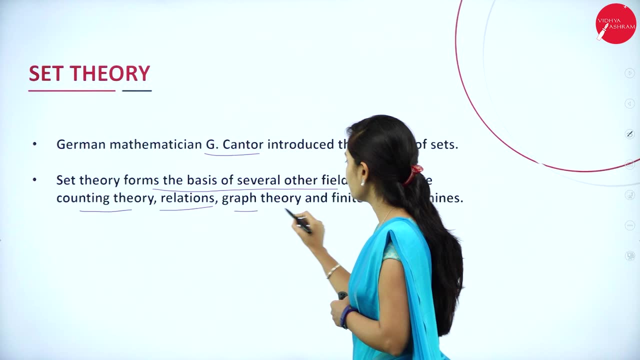 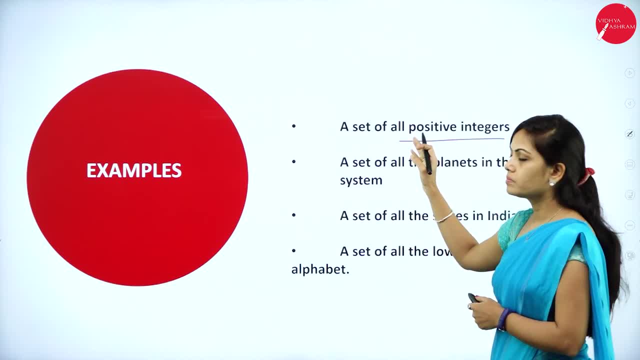 And set theory forms the basics of several other fields of study, like counting theory, relations, graph theory and finality. So we can take this example: set of all positive numbers. that means plus 1,, 2,, 3,, 4, 5, etc. 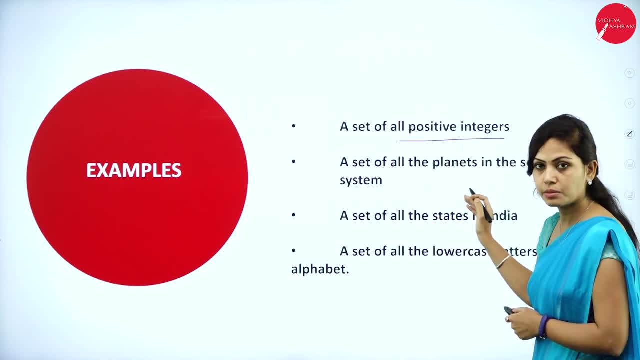 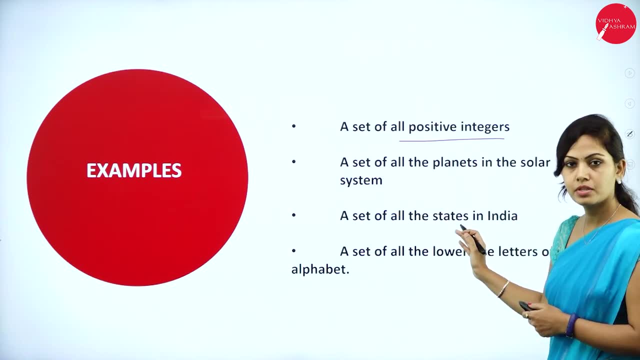 and set of all the planets in the solar system, So it is a unordered collections of objects, and a set of all the states in India. So it is a collections of objects. So we can call: this is the set elements and a set of all the lowercase letters of the alphabet. 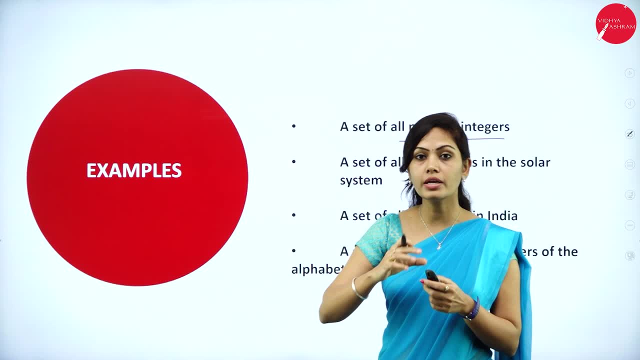 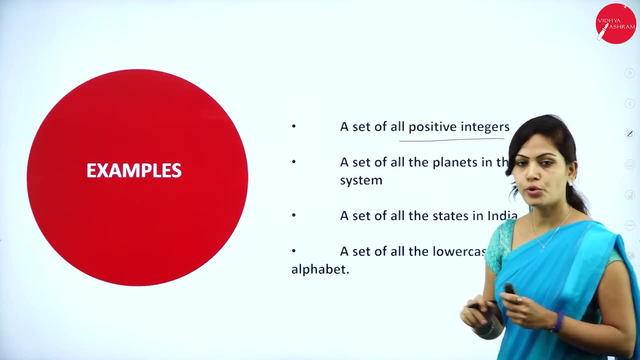 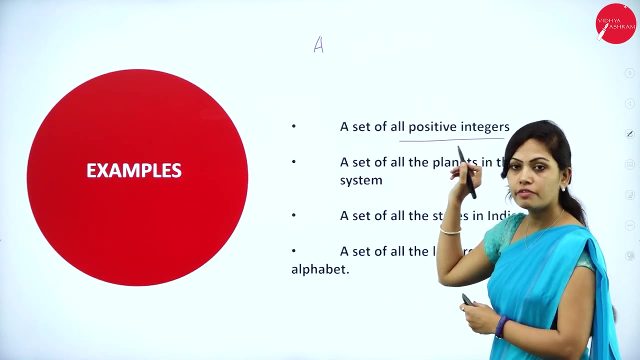 So it is a unordered collections of objects, or it is a well-defined objects, or also known as elements, And keep in mind, set can be denoted by a capital letters, A, B, C, etc. So, example: a set of all positive integers. So I will list out all the positive integers. 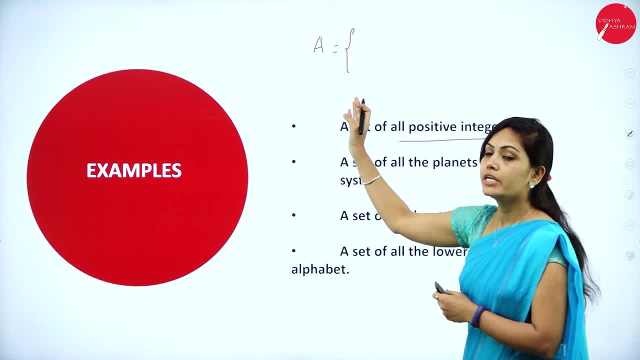 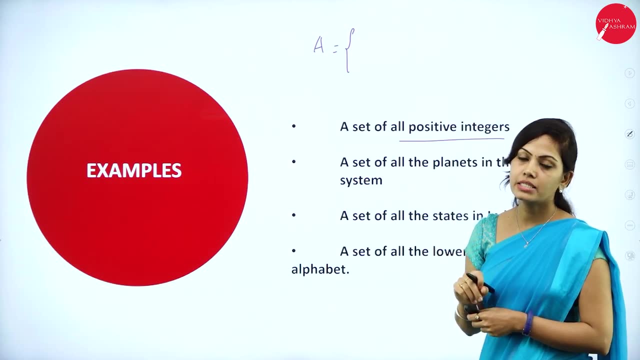 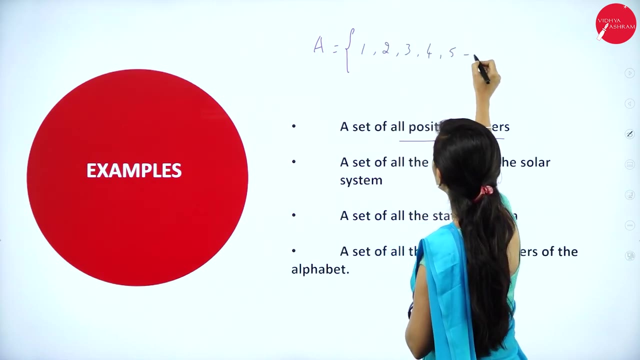 Within a flower bracket, So set can be denoted by a capital letters within the flower brackets. I can mention all the sets elements. So example: set of all positive integers, So 1,, 2,, 3,, 4, etc. So this is one set. 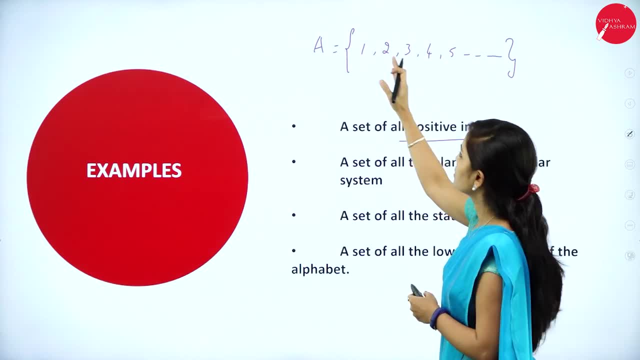 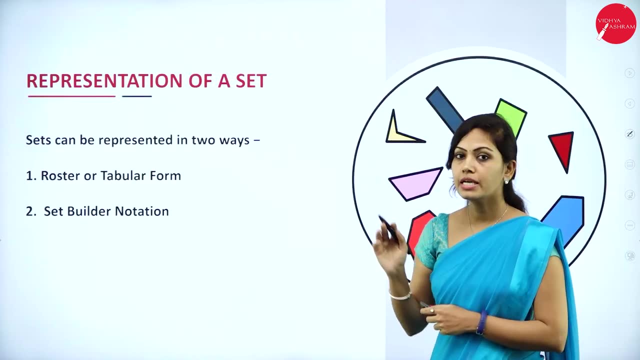 Set can be denoted by a capital letters within the flower brackets with comma. So this is one set, So this is one set. So this is an example for set. And set can be represented by: is roaster or tabular form or set builder notation. 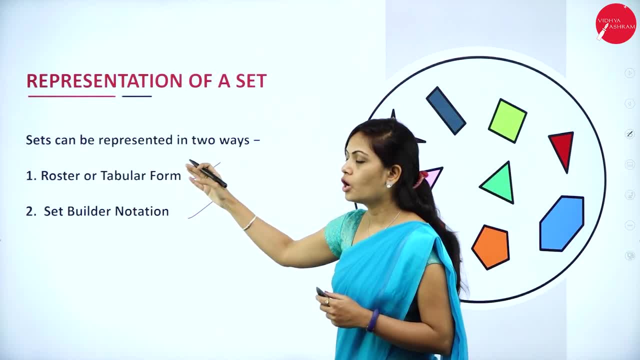 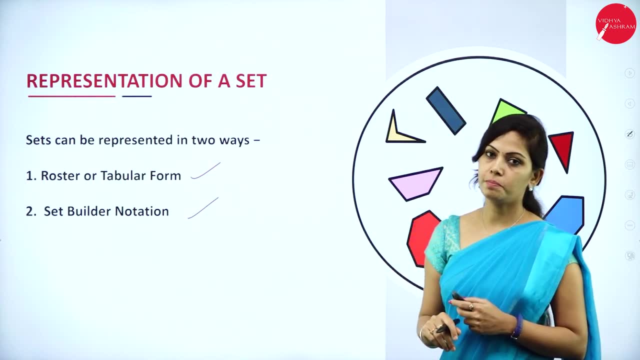 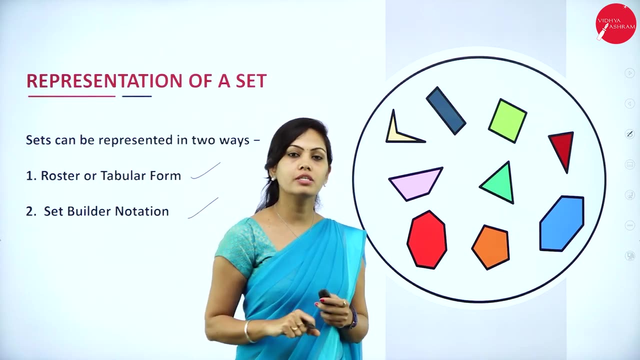 Very important question for two marks. What is roaster form? or you can expect, set builder form. So what is this? roaster form or set builder form? So the representation of sets can be divided into two parts, That is, set builder form and roaster form or tabular. 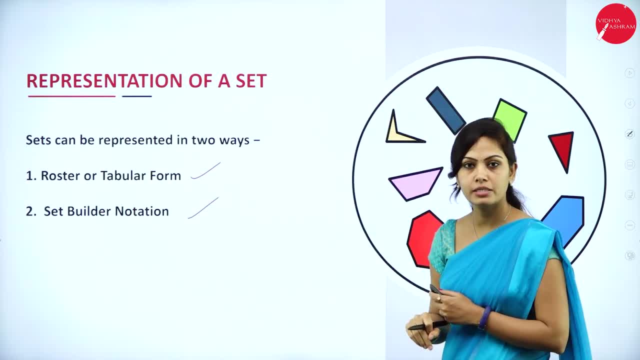 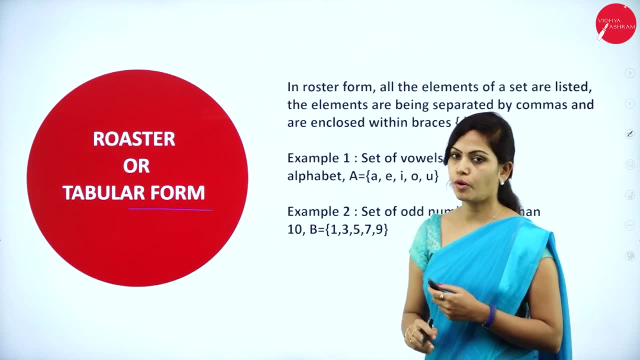 So what is this roaster form and set builder form? So first one is roaster or tabular form. What is this roaster form? In roaster form, all the elements of a set are listed. The elements are being separated by commas and are enclosed within flower braces. 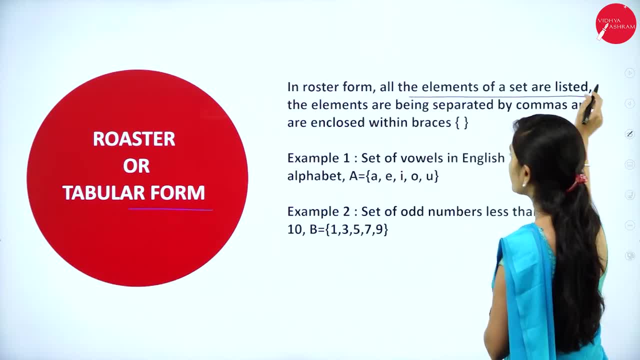 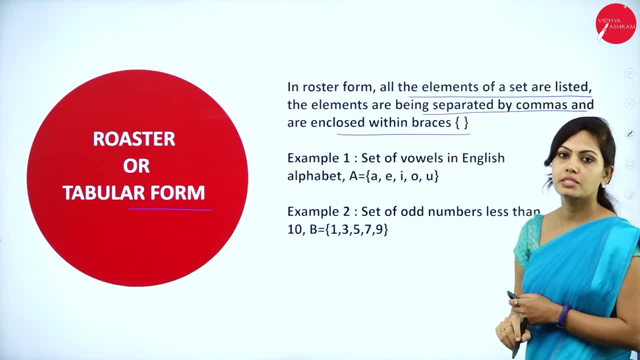 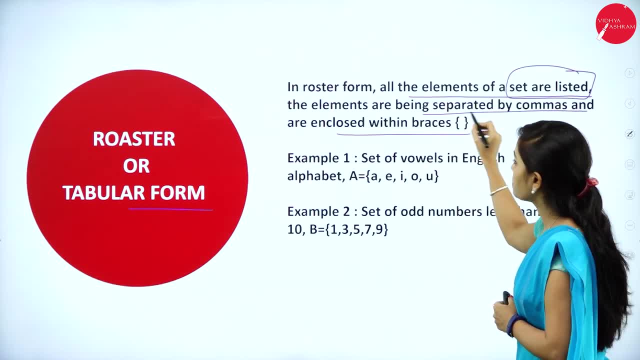 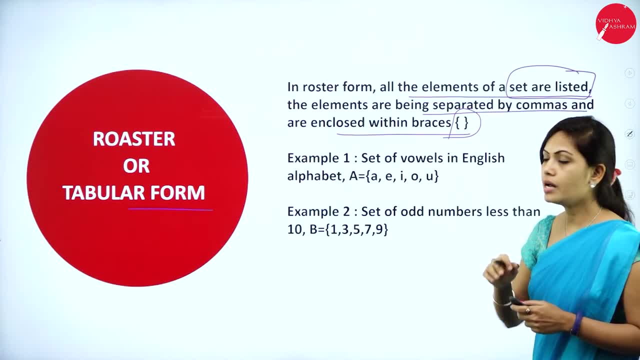 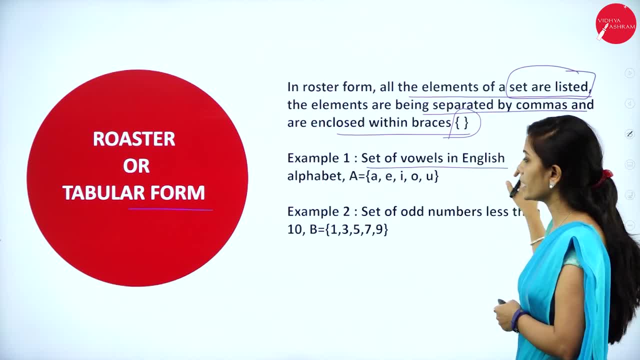 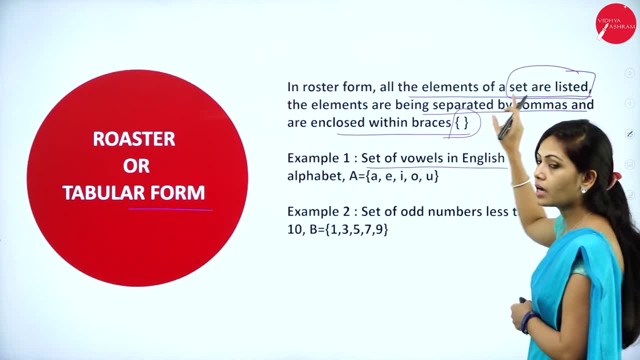 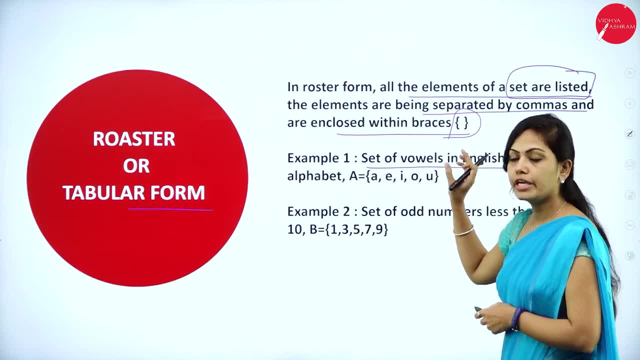 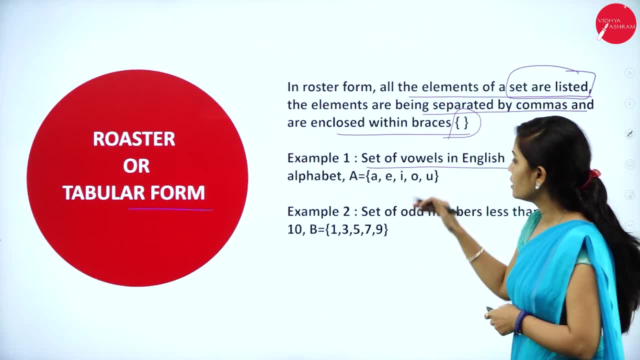 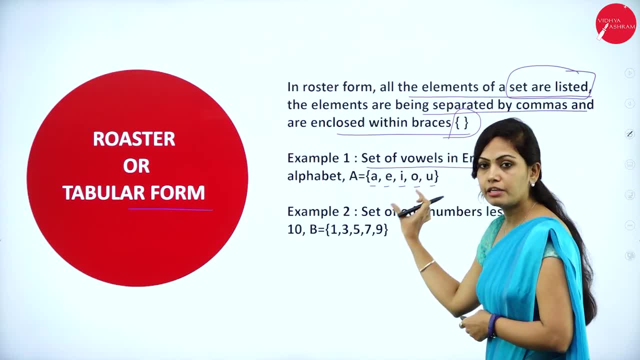 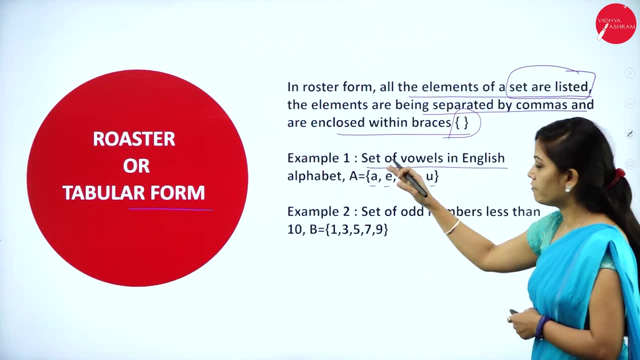 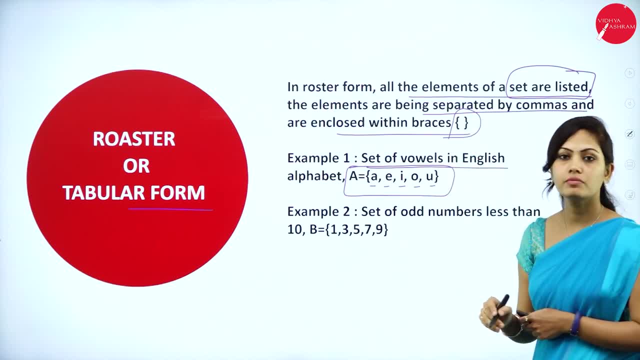 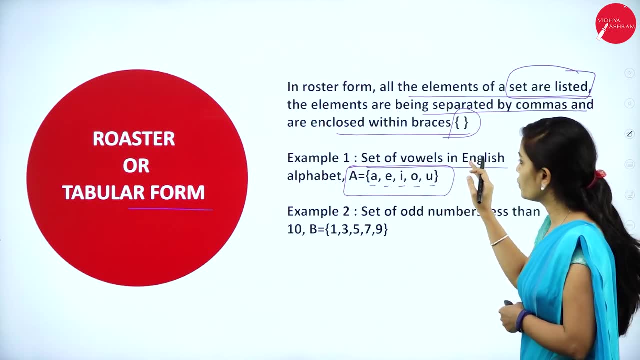 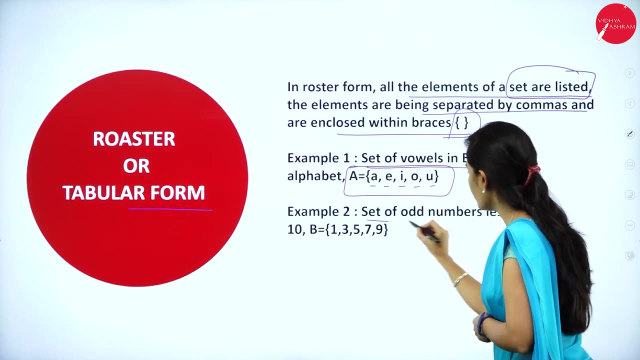 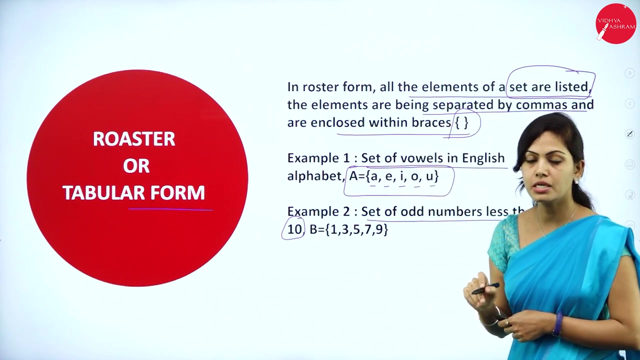 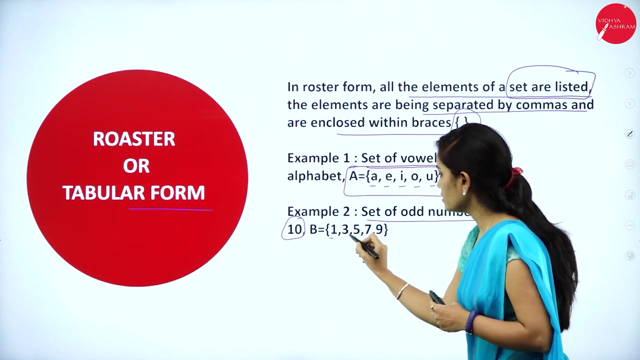 alphabet. So have listed all the set of ovals in English alphabet. That is A is equal to A, E, I, O, U, enclosed within braces and separated by a comma. So another example. I have one statement here: set of odd numbers less than 10.. How many odd numbers are there? That is 1, 3, 5, 7 and 9.. These 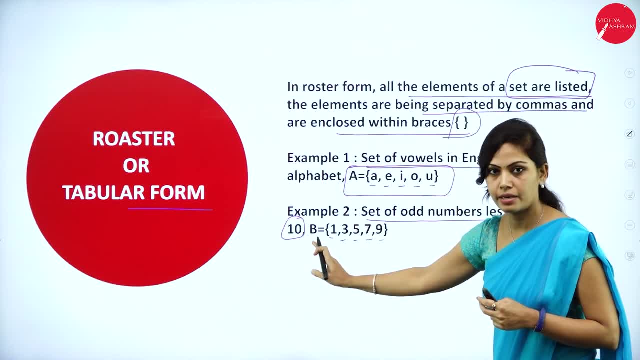 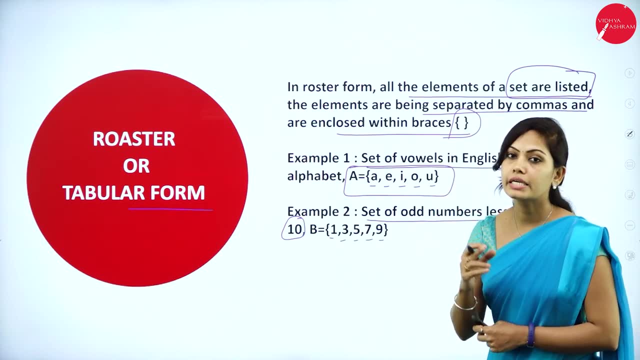 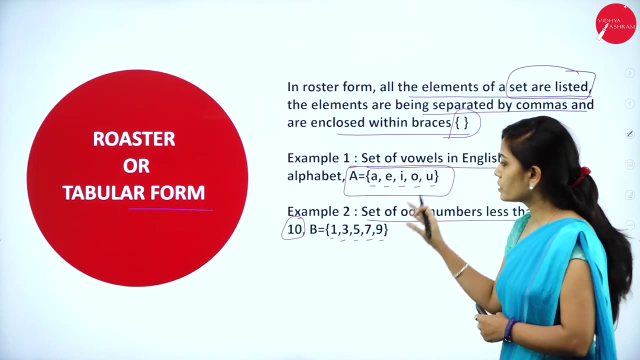 are the odd numbers less than 10.. So here I have one statement. This statement have converted as roaster or tabular form. 9 enclosed within flower brasses. So this is called as roaster or tabular form. So we have. 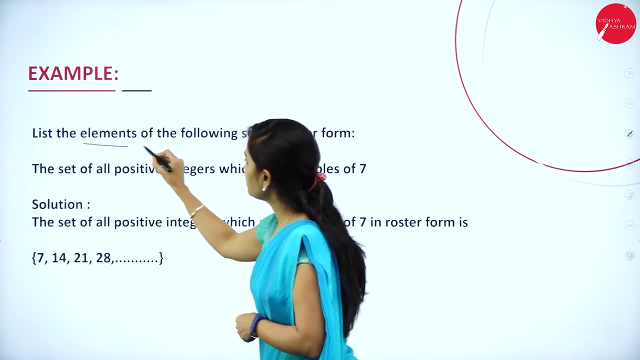 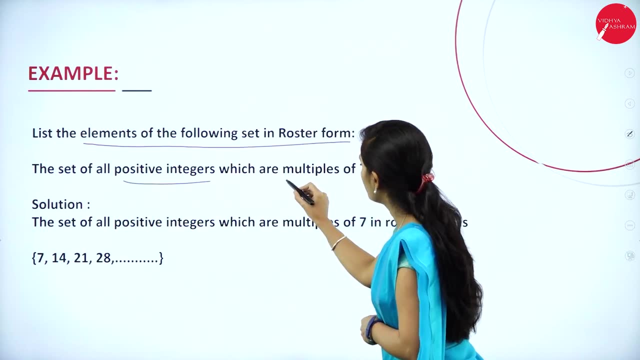 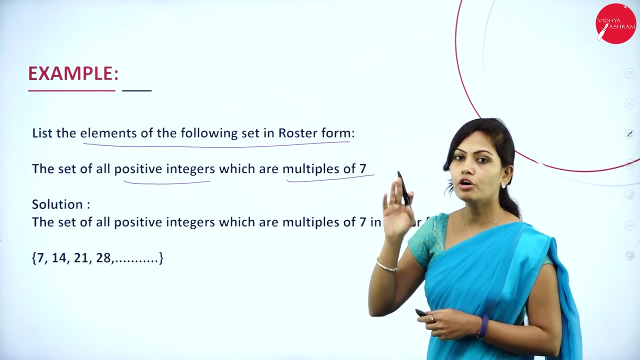 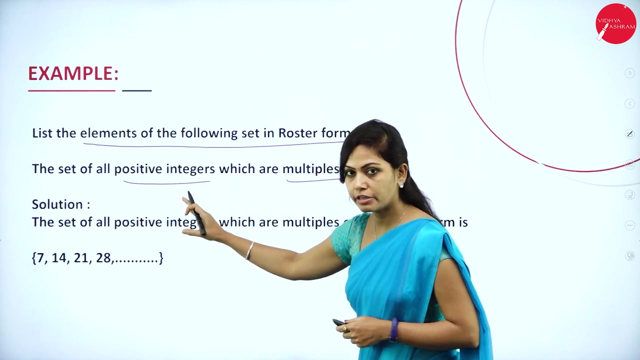 another example for roaster method: List the elements of the following: set in roaster form: The set of all positive integers which are multiples of 7.. So how to write this statement in roaster form: Set of all positive integers which is multiples of 7.. So here I have listed. 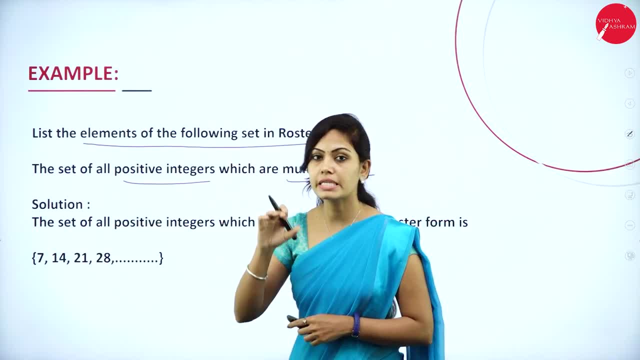 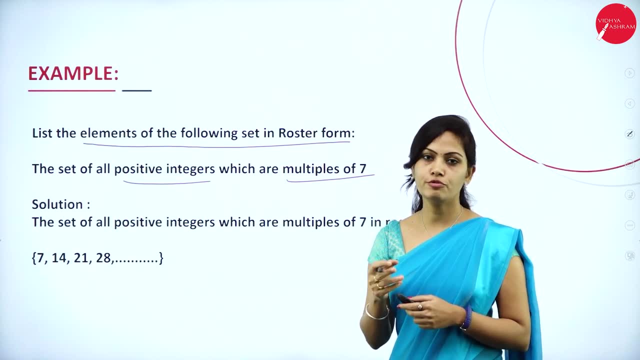 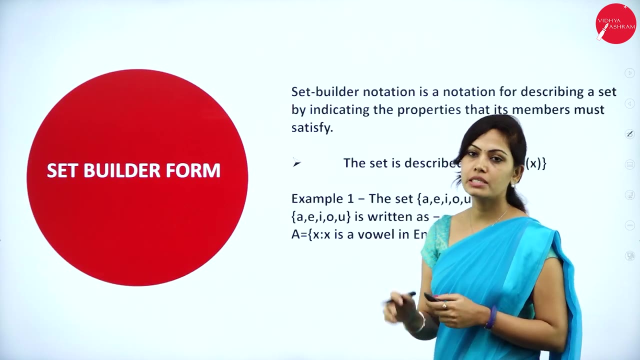 the elements. I have listed the set elements in roaster form So you can give this example for roaster form or tabular form. Roaster form is also known as tabular form And next representation is set builder form. So set builder notation is a. 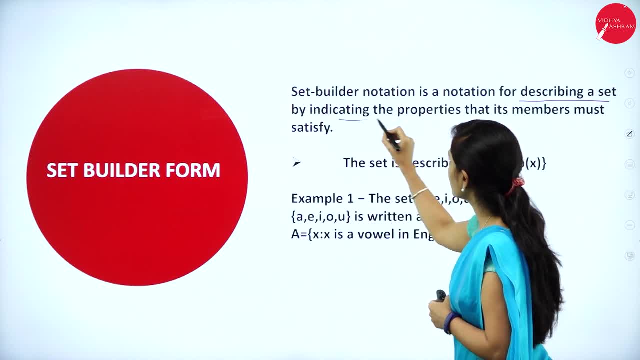 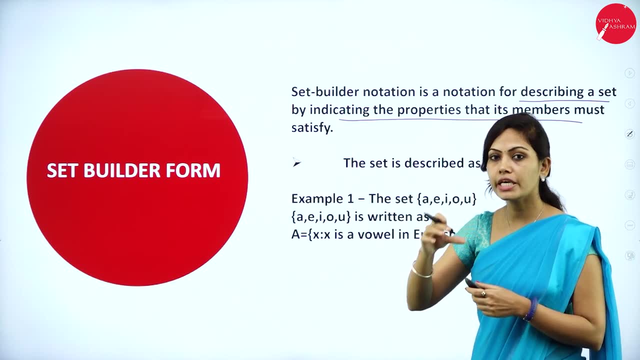 notation of set builder form. So set builder notation is a notation of set builder form. So set builder notation is a notation for describing a set by indicating the properties that its members must satisfy. So here, instead of listing the elements, here I have to give the 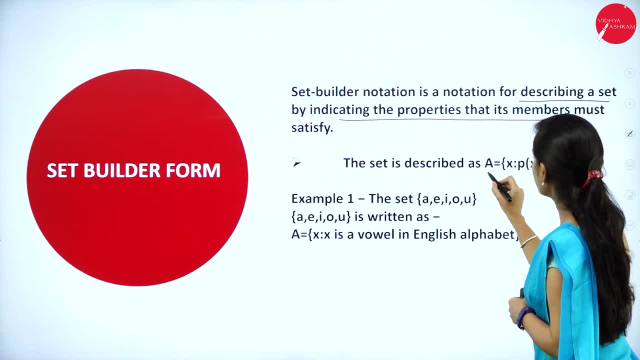 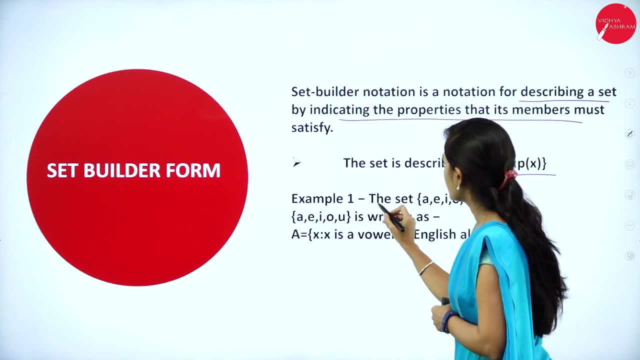 statements. So here the set is described as a- is equal to x, such that p of x- I will take this example- The set a, e, i, o, u- Here I have the list of elements that I will list. So here I have the. 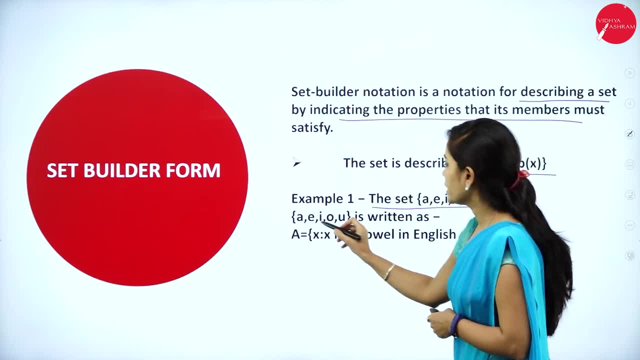 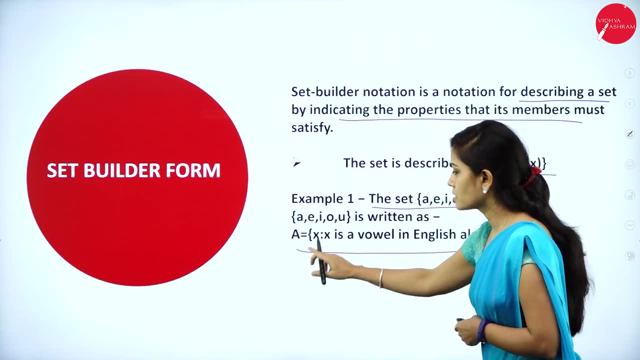 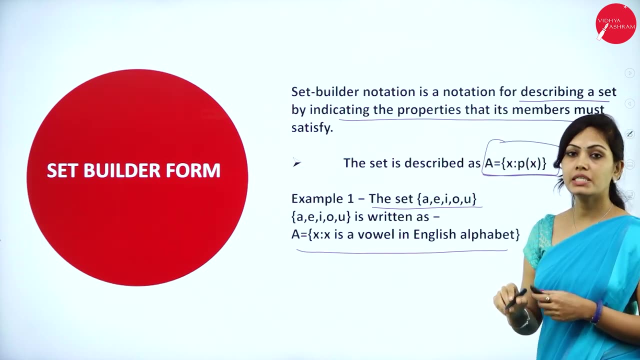 statement that I will convert it into set builder notation. A, e, i, o, u is written as in set builder form, So a is equal to x, such that x is a oval in English alphabet. So this is a syntax for representing a set builder form, That is, set: a is equal to x, such that p of x. So here I will mentioned the statement of a given. 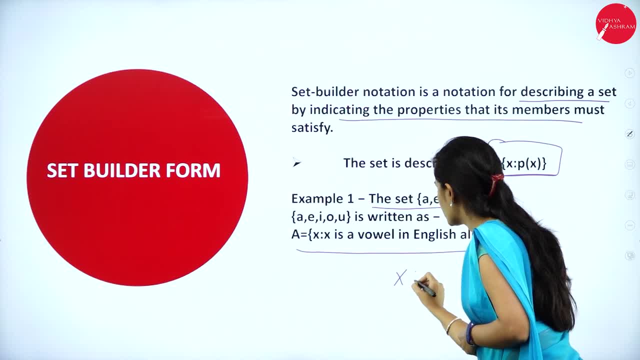 set x, such that p of x- Here I will mention the statement of a given set x- 0- is equal to p of x. So in this case I am writing- and I need to convert the whole list until by the colon stands for such that x is a probable in English alphabet, Instead of writing: 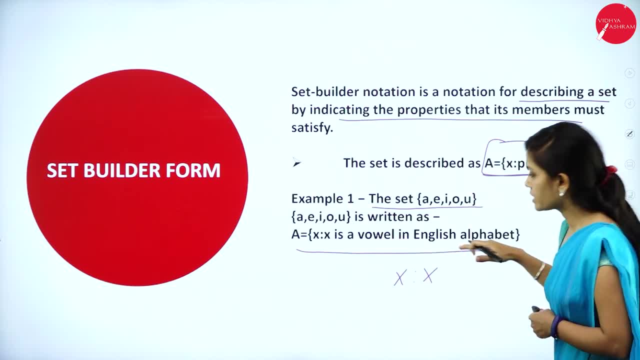 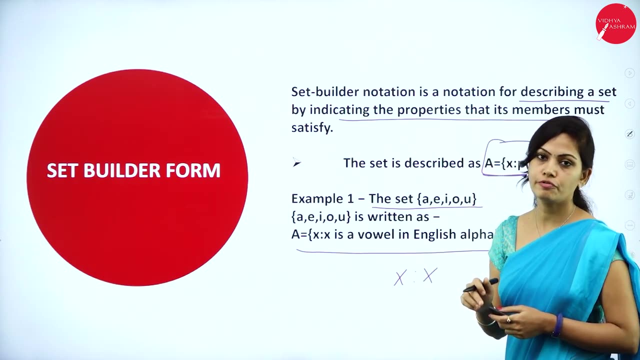 instead of listing the elements, I am writing the statements in set builder form. It's very simple concept: In set builder form, we are not listing the elements. So, instead of listing the elements, we are giving the statements for a given set of elements In roaster form. we are: 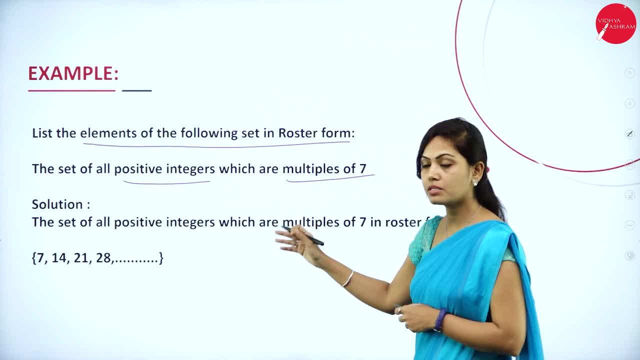 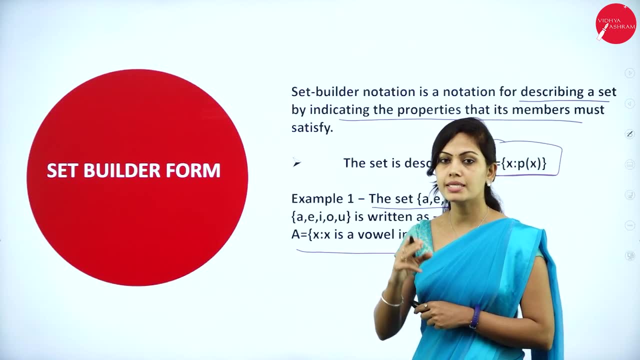 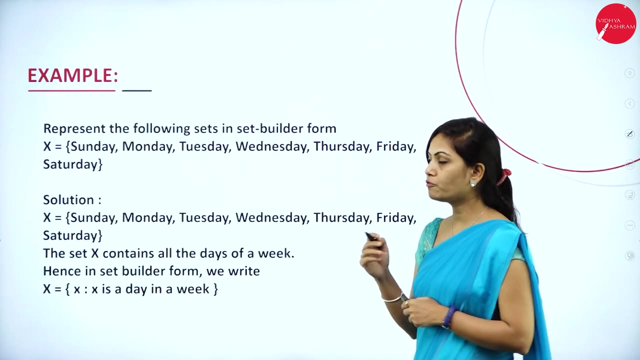 listing the elements Instead of writing the statements. we are listing the elements in roaster method. So in representation of sets we have two methods, that is, roaster form or tabular form. Also we have set builder form. So another example for set builder form: x is equal to Sunday. 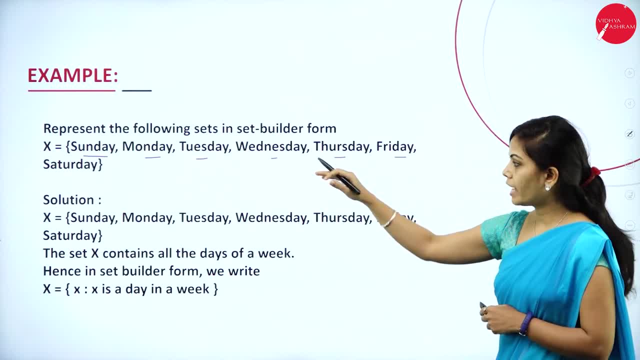 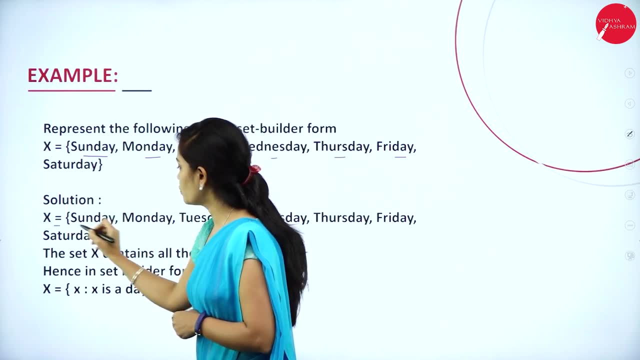 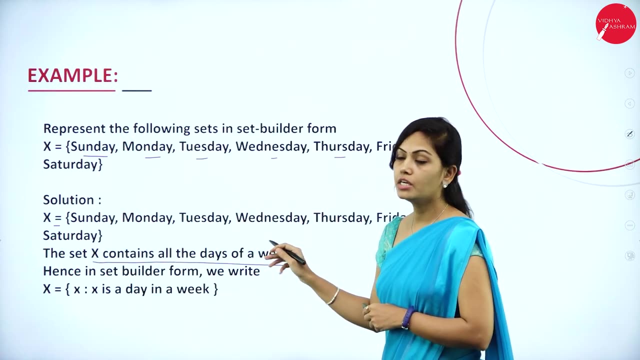 Monday, Tuesday, Wednesday, Thursday, Friday and Saturday. We have list of elements here, So how to write it in a statement called set builder. form X is equal to Sunday to Saturday. The set x contains all the days of a week. So instead of: 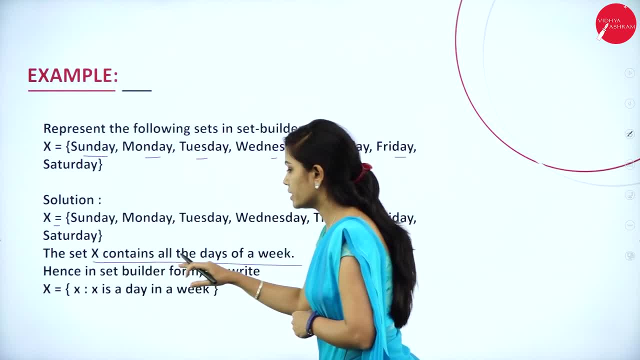 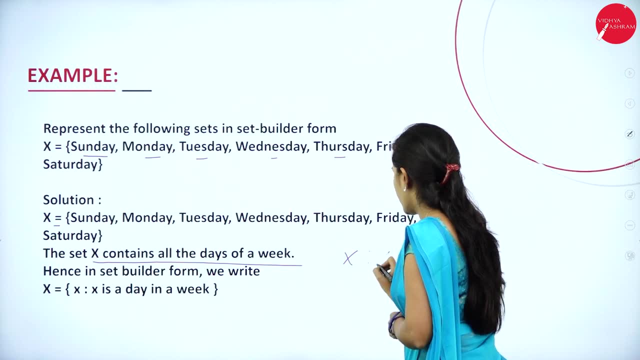 listing the set elements. you can write: x contains all the days of a week. So how to write this in a set builder form, So x, such that x is a day in a week. So in set builder form instead of. 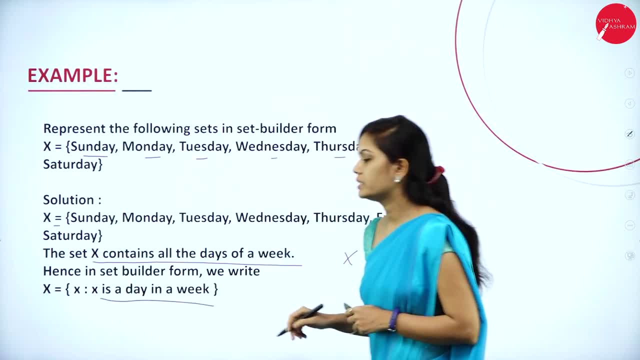 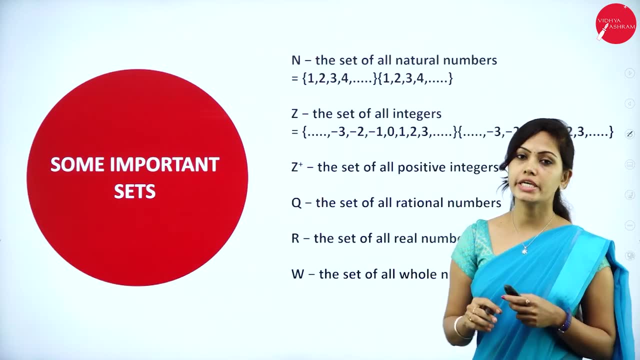 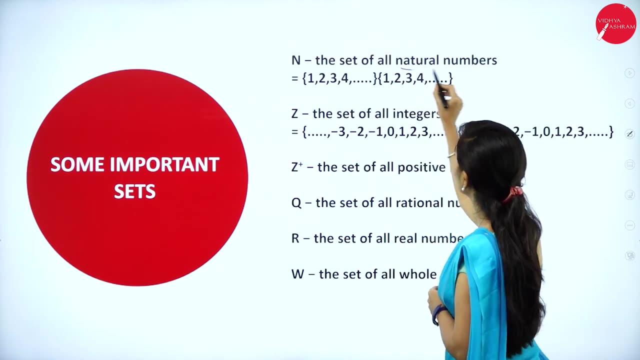 listing the elements. you can write the sentence. So this is your example for set builder form. So next concept is some important sets. So in set theory we have some important sets. So n is called as the natural numbers. So 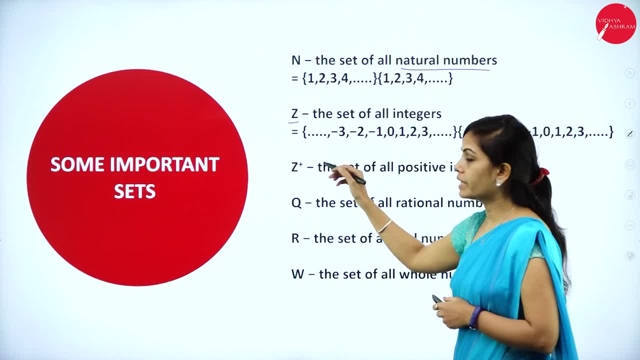 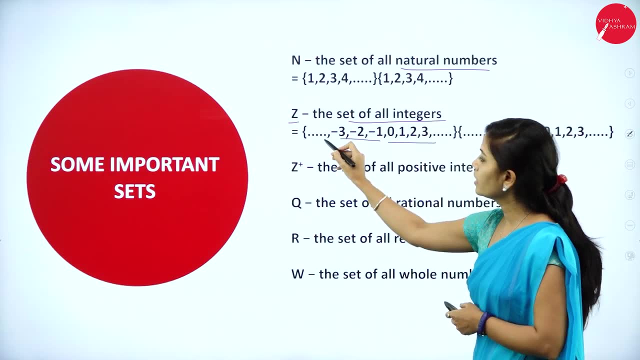 n is equal to 1,, 2,, 3,, 4, etc. And z is called as set of all integers. Set of all integers means it can be positive integers or negative integers, So we can represent it by z. 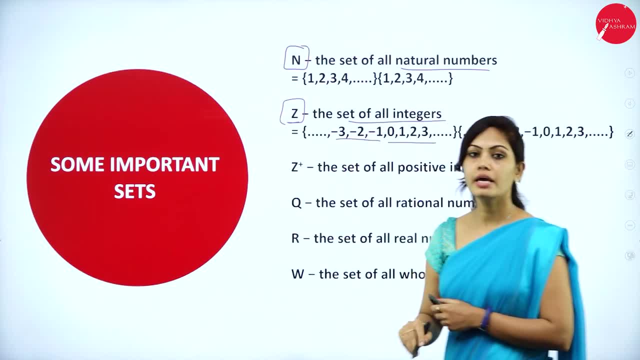 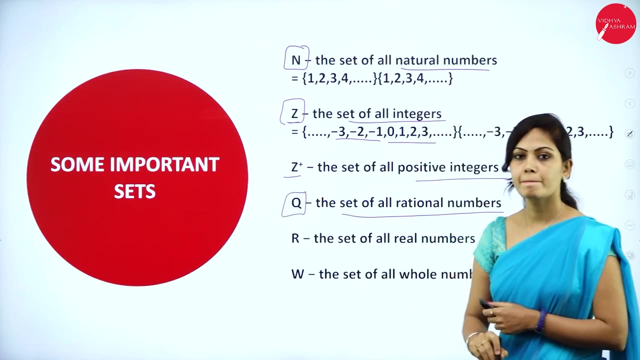 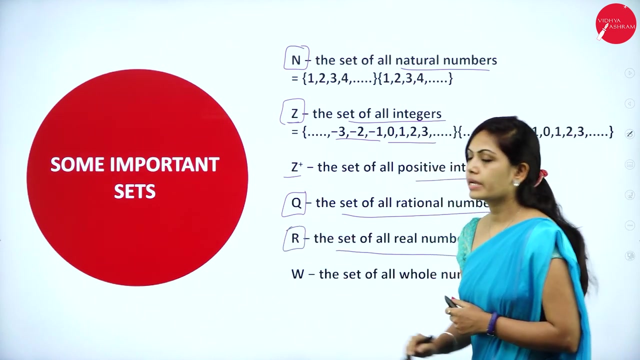 So natural number is represented by n And z plus. the set of all positive integers is represented by z plus And the set of all rational numbers is represented by q. And the set of all real numbers, set of all real numbers, is represented by capital R, And the set of all whole numbers is: 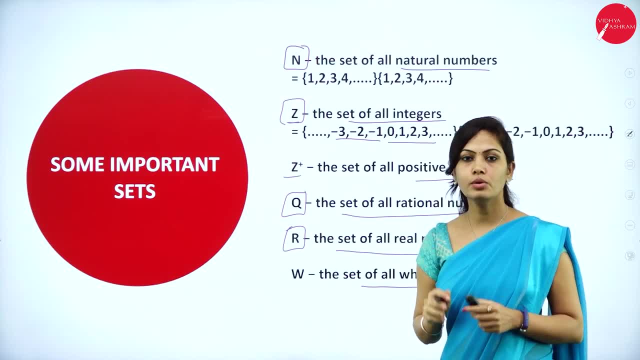 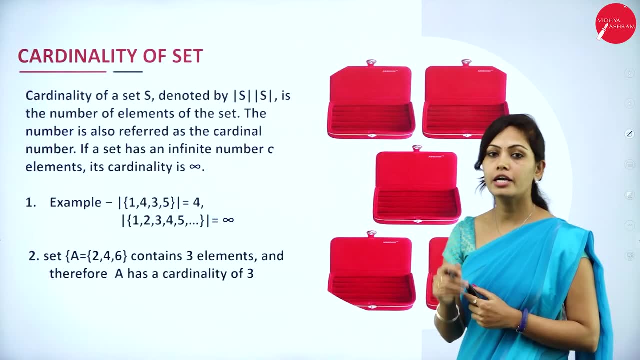 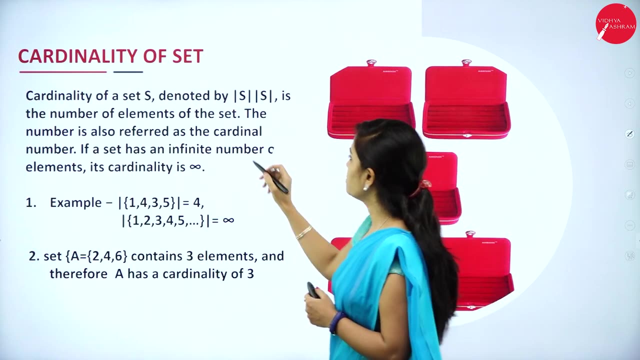 represented by w. So these are the common, very important sets we are using in set theory. So next important concept is cardinality of a set. So what is this cardinality of a set? Cardinality of a set is denoted by mod s. So what is this cardinality of a set? It is represented. 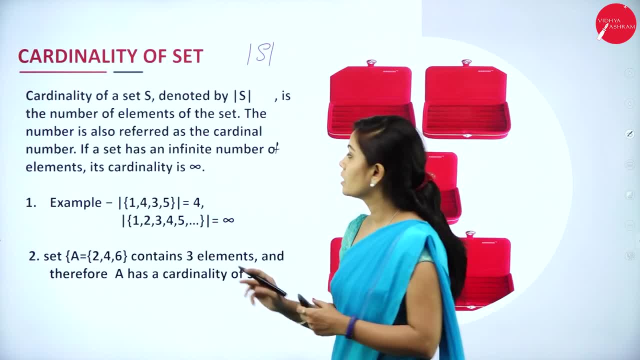 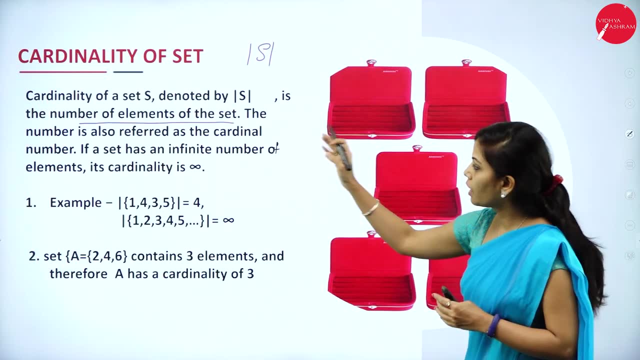 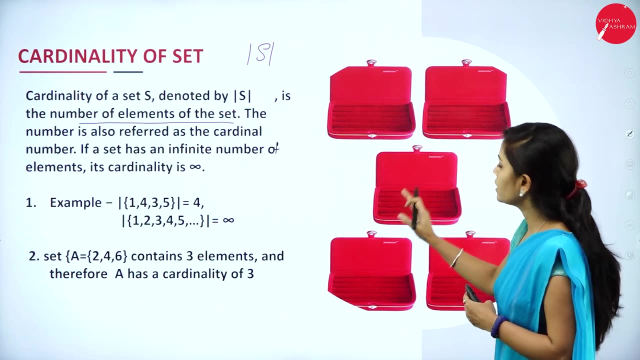 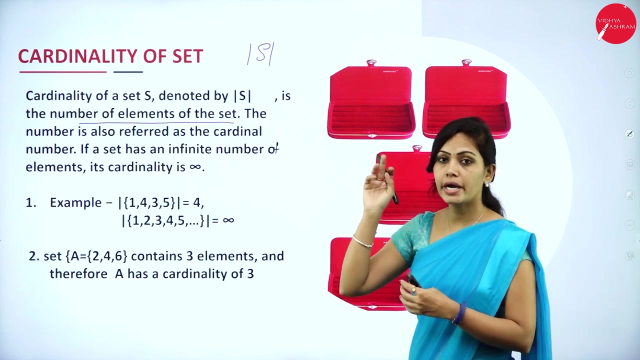 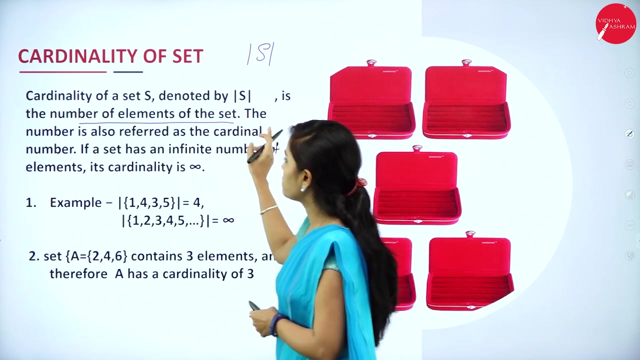 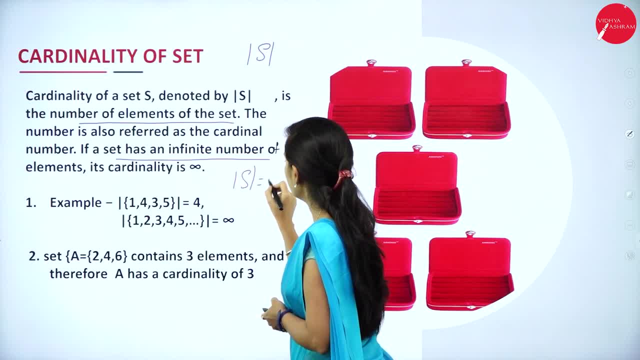 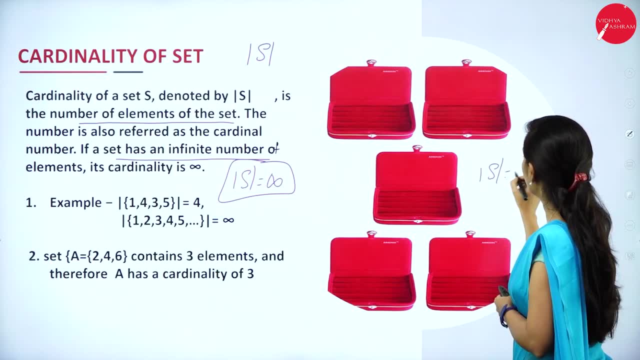 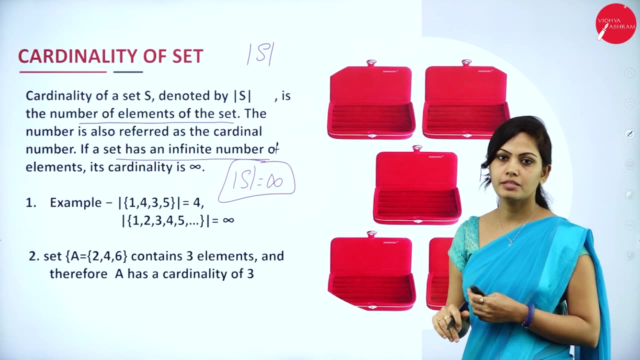 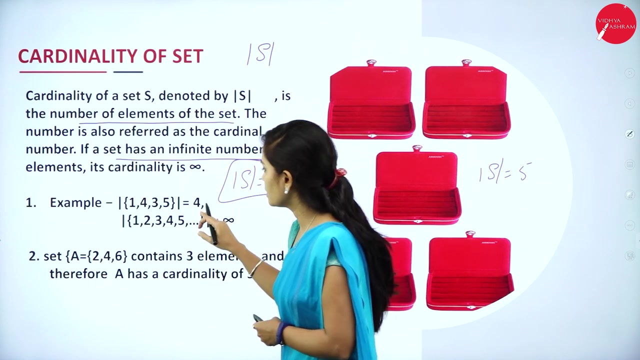 by the symbol mod s, is equal to infinity. So here I can write: the cardinality of this set, mod s, is equal to 5.. We have 5 number of elements. This is called as cardinality of a set. Examples: 1,, 4,, 3, 5 is equal to 4.. So how many number of elements are there? 1,, 2,, 3,, 4.. So we 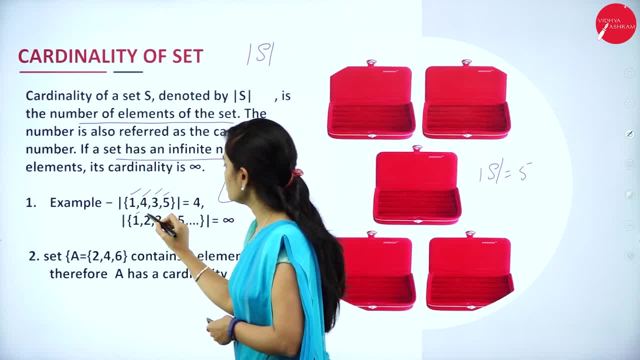 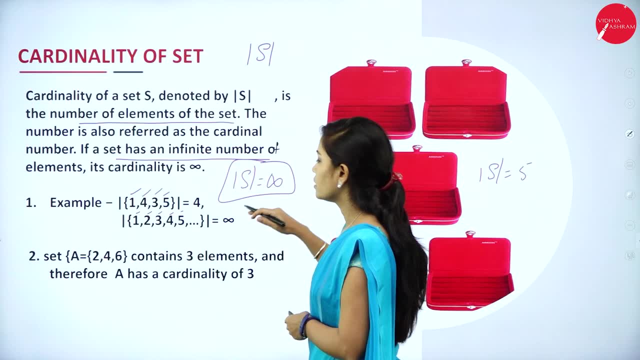 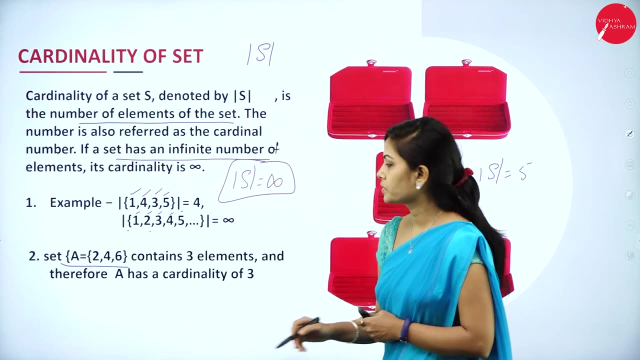 have 4 number of elements and 1,, 2,, 3,, 4,, 5,, etc. etc. So how many number of elements are there? We have infinity number of elements. Next example is set: a is equal to 2,, 4,. 6 contains 3 elements. 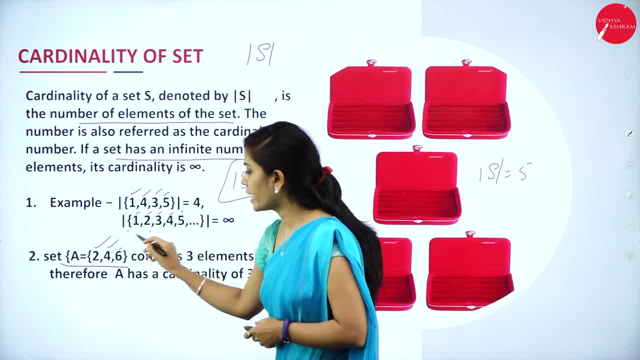 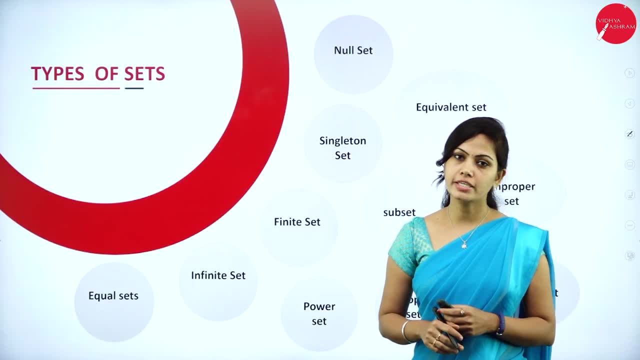 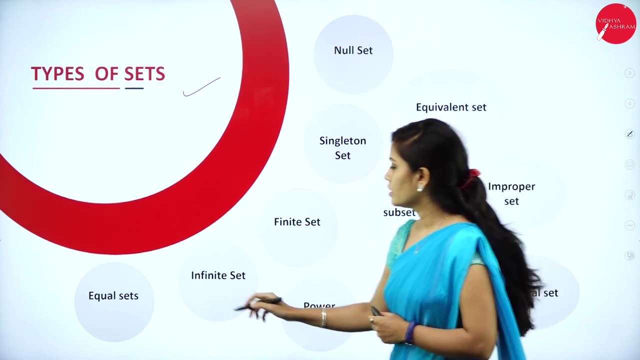 Is it right? So here we have 3 elements: 2,, 4 and 6.. The cardinality of this set is equal to 3.. And next important concept is types of sets. So we have different types of sets. that is null set. 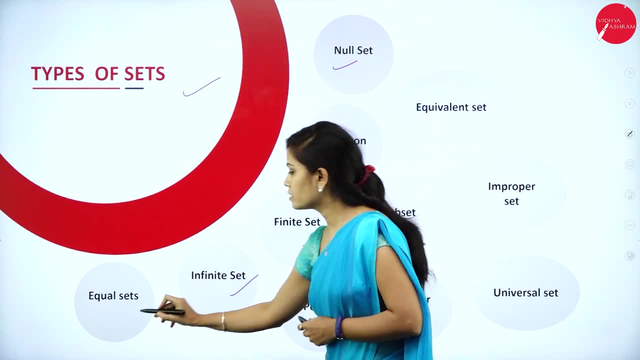 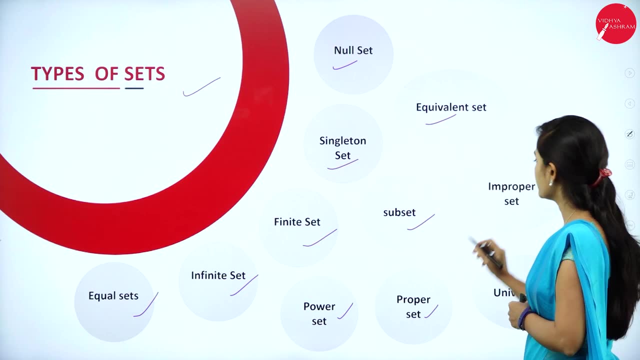 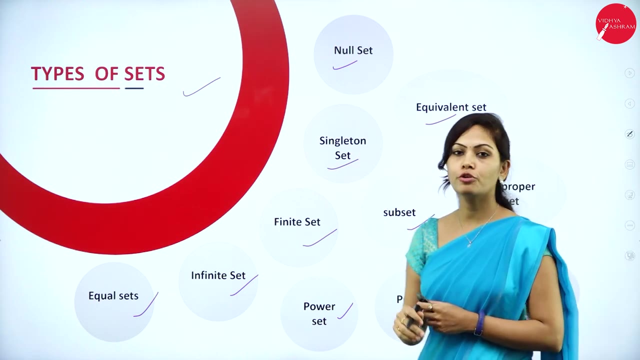 singleton set, finite set, infinite set, equal sets and equivalent sets, subset, power set, proper set, improper set and universal set. So we have different types of sets. Let's see how many sets are there. So we have 3 sets of sets. So we have 3 sets of sets. 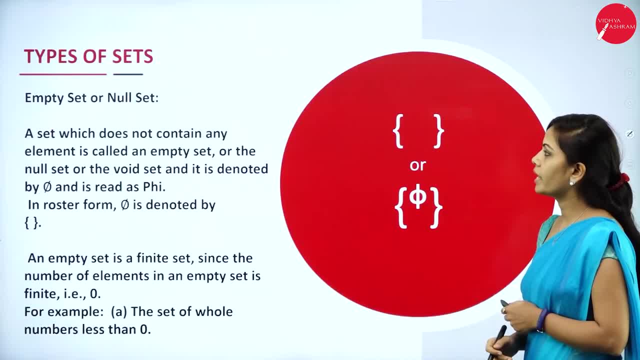 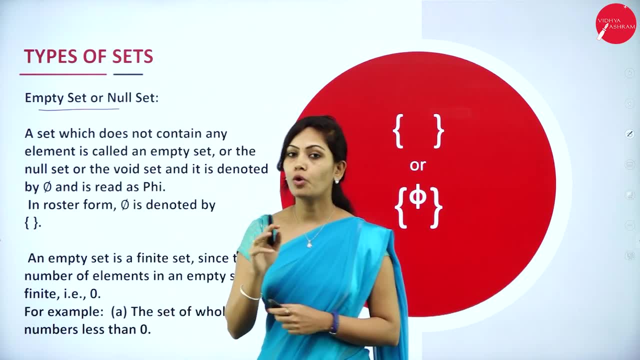 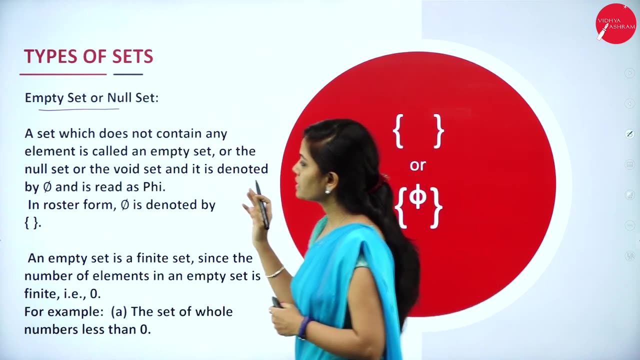 Let us understand one by one. So first type: we have null set. Null set is also known as empty set. To Mark's question: what is null set? Give an example. Null set is also known as empty set. So what is the definition of null set, A set which does not contain any element? 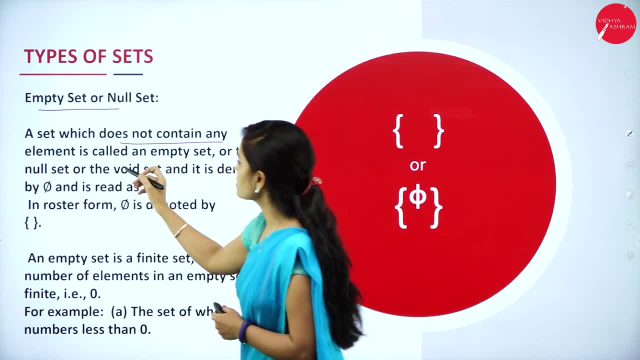 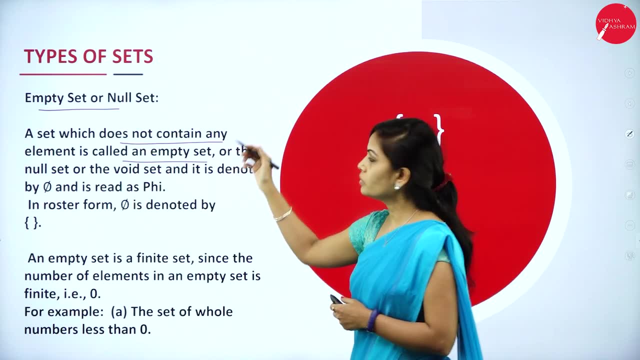 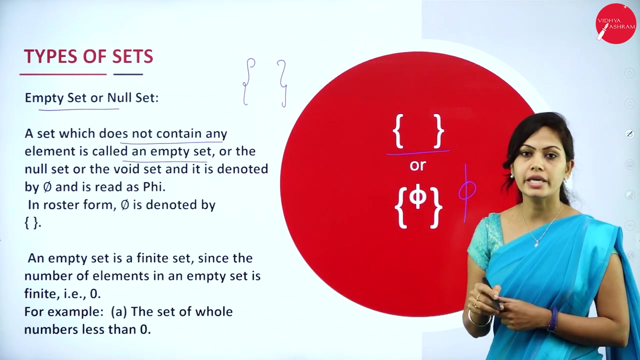 A set which does not contain any element means it is called as empty set or null set. It does not contain any elements, So it is an empty. The set it does not contain any element means we can call it as it is an empty set or we can represent it by phi. 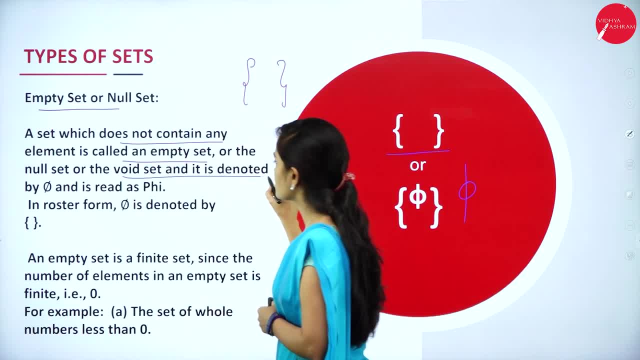 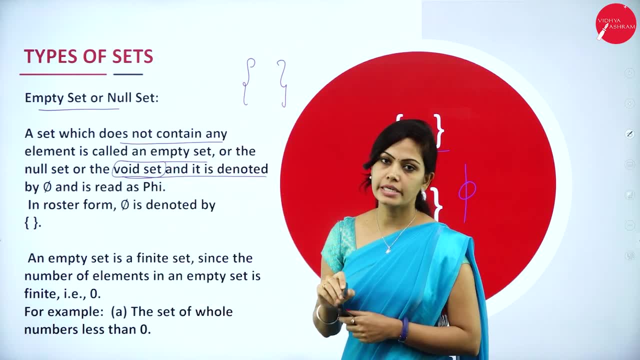 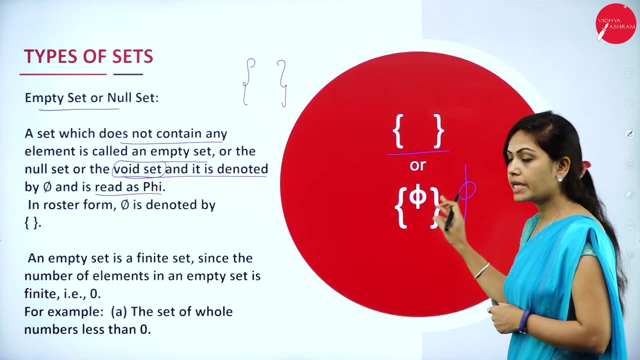 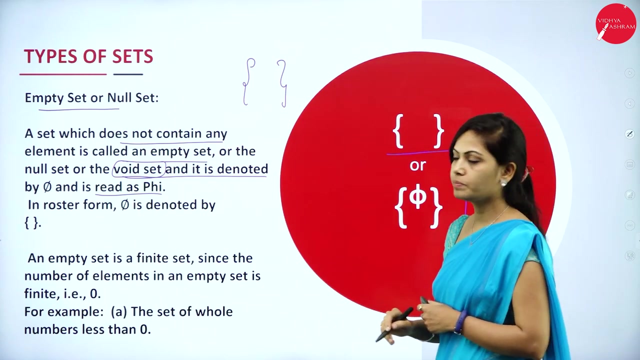 Or the null set or the void set, and it is denoted by phi symbol. Null set also known as empty set, or void set also, And it is read as phi. This symbol is phi symbol. If a set which does not contain any element means we can represent, it, is this null set. 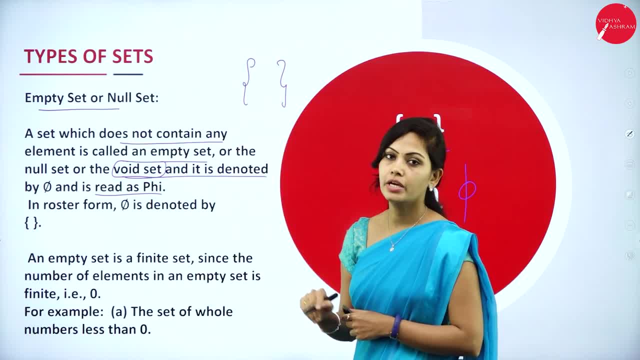 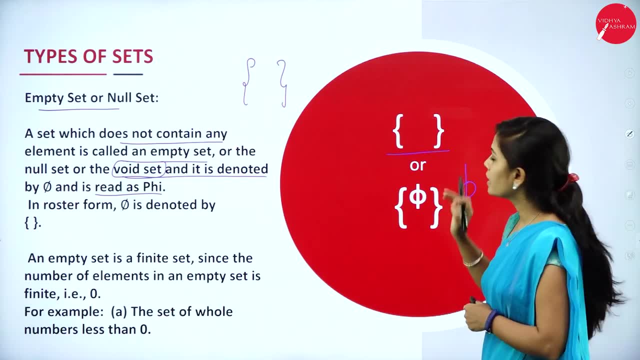 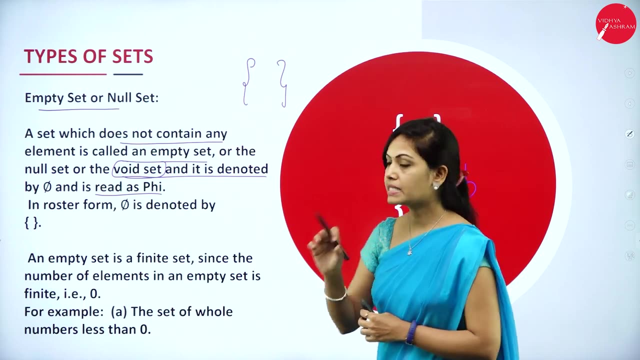 An empty set is a finite set. An empty set is called as finite set. So because we can call it as it is a null test. There is no number of elements means we can call it as it is a finite set. So, empty set, This is one empty set. This empty set is called as a finite set. 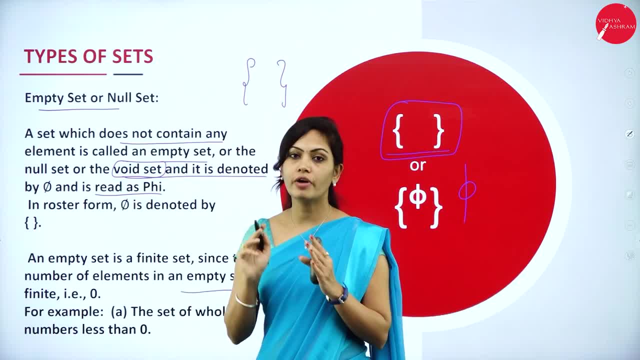 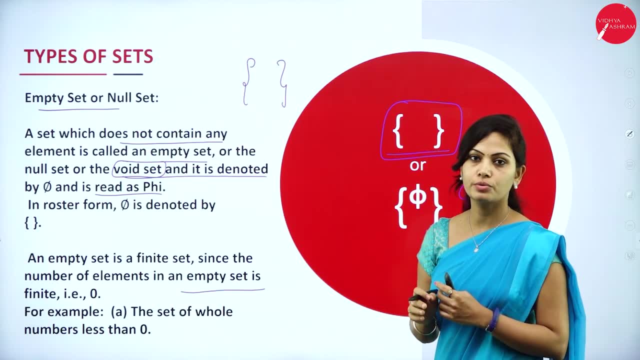 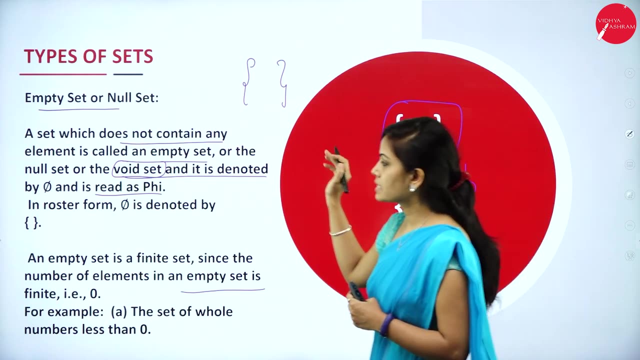 Since the number of elements in any empty set is finite, that is zero. Here there is no number of elements, so I can call it as is a finite set also. So null set is also known as empty set or void set. If a set which does not contain any element is called as null set or empty set, 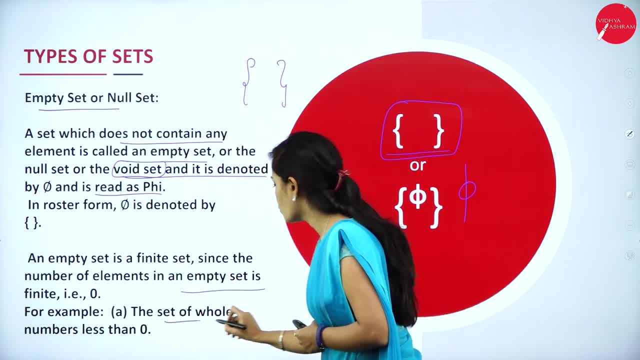 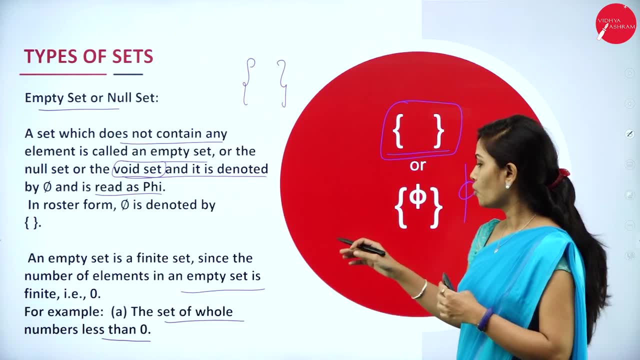 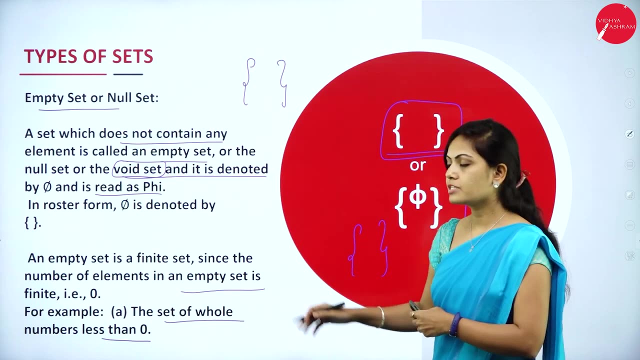 Example: The set of whole numbers less than zero. It is obviously not possible. The set of whole numbers less than zero. So the set value is this: null. There is no whole numbers less than zero, right? So it is an empty set. So this is one best example for null set. 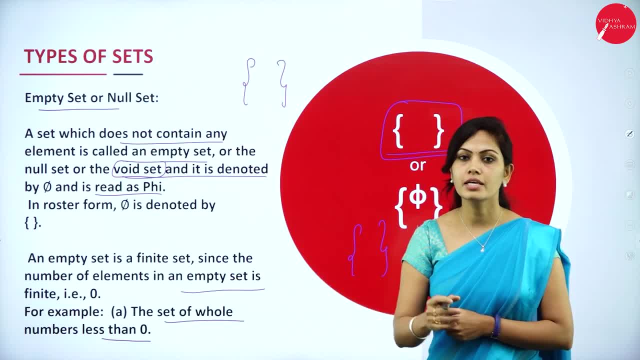 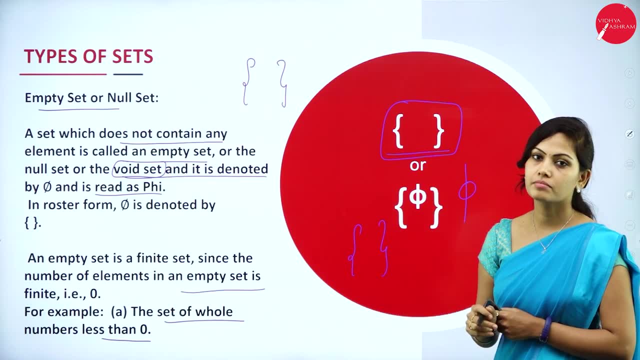 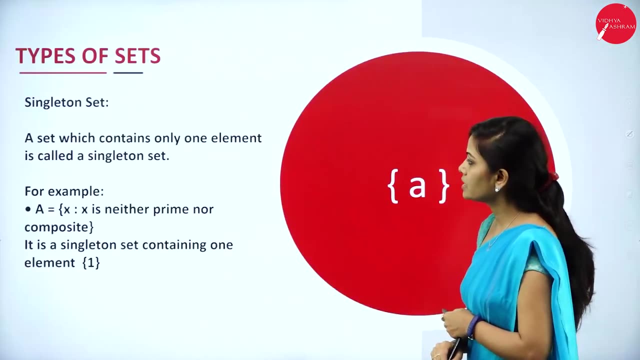 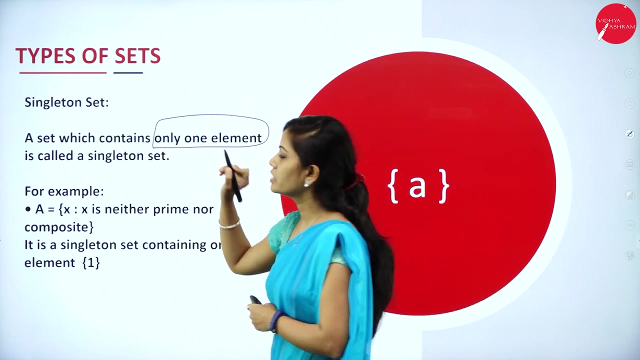 The set of whole numbers less than zero, Zero, Clear. So this is called as null set or empty set or void set. So it is represented by the symbol called phi. And the next type is singleton set. Singleton, A set which contains only one element, is called as singleton set. 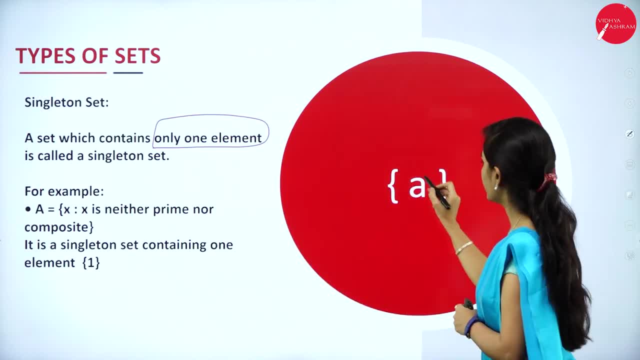 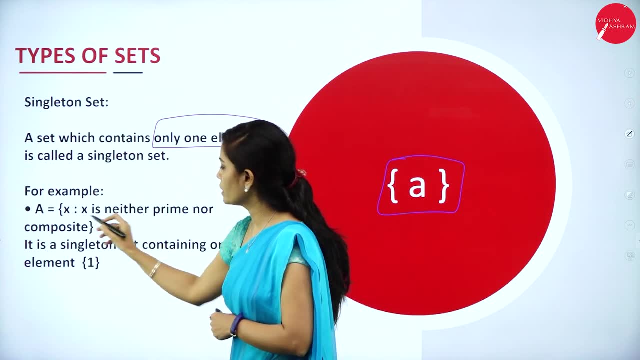 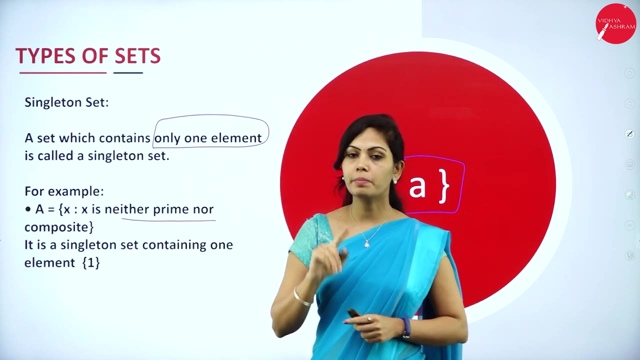 A set contains only one element. Set contains only one element is called as singleton set. So example: We have one statement, X, such that x is neither prime or composite. So we have only one prime or composite number. that is one. So answer is one. 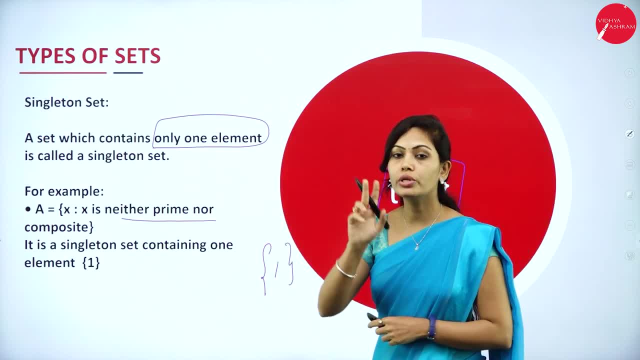 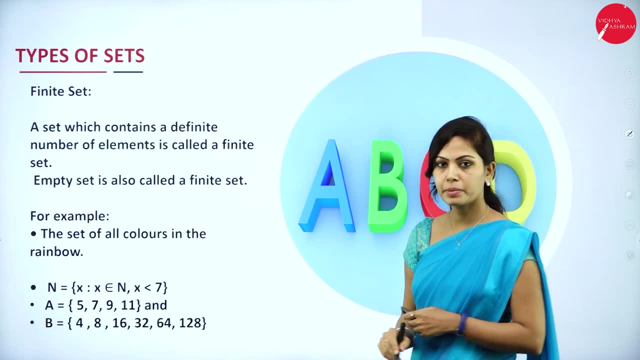 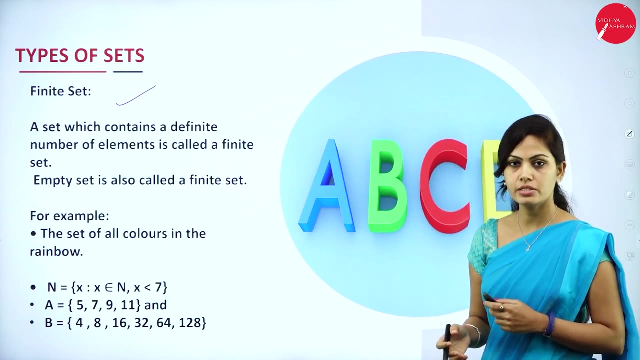 So singleton set means a set which contains only one element. Only one element is called as singleton set And next type is Finite set. What is this finite set? We have number of elements in a set. So if you are able to count the set elements, that is called as finite set. 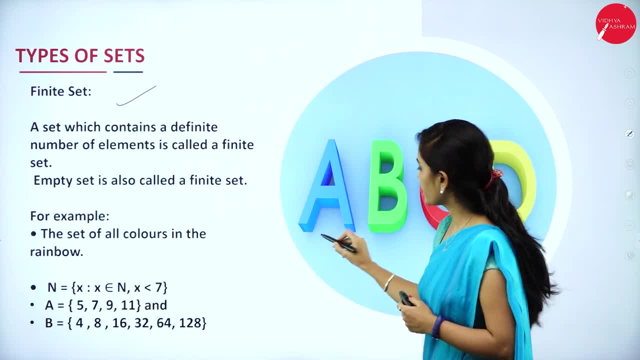 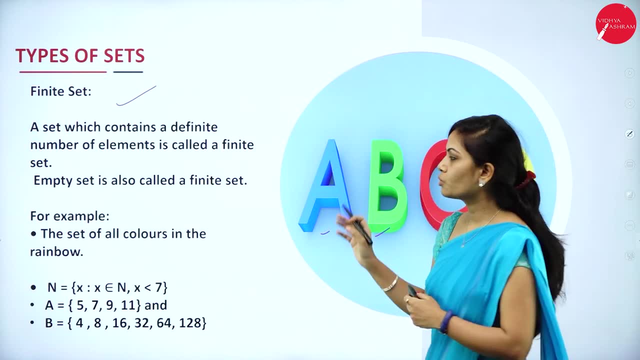 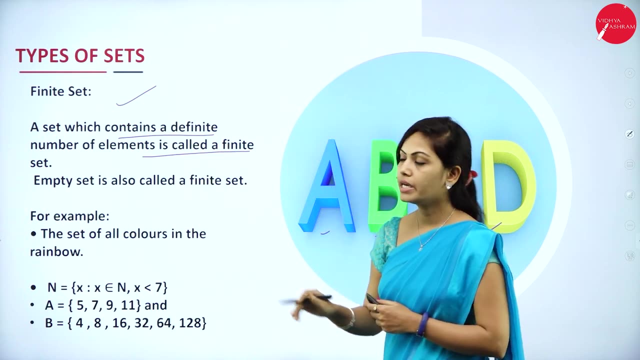 So here I have one set elements. I can count this: elements A, B, C, D Right. So this is a finite set. So what is the definition? A set which contains a definite number of elements is called a finite set. A set which contains a definite number of elements. 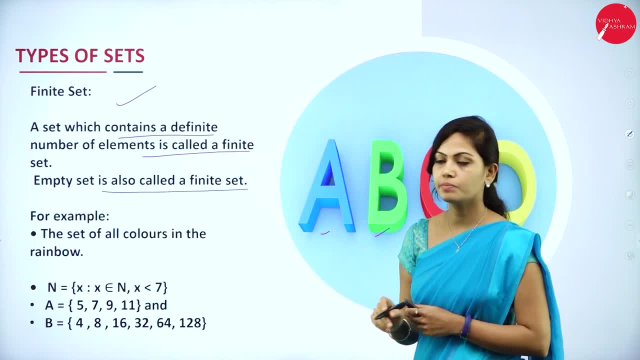 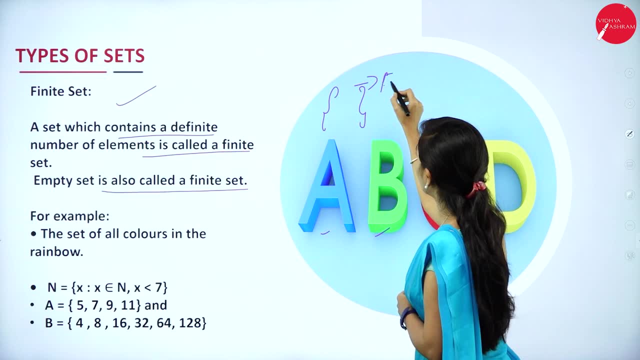 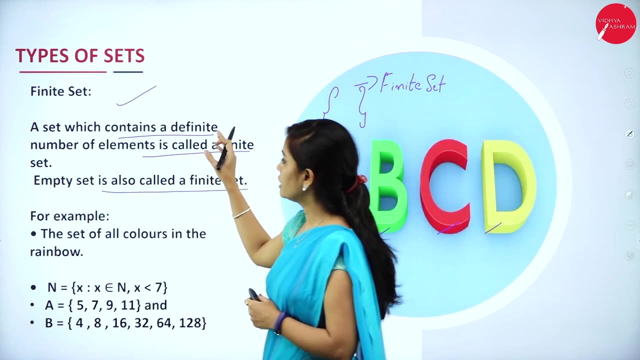 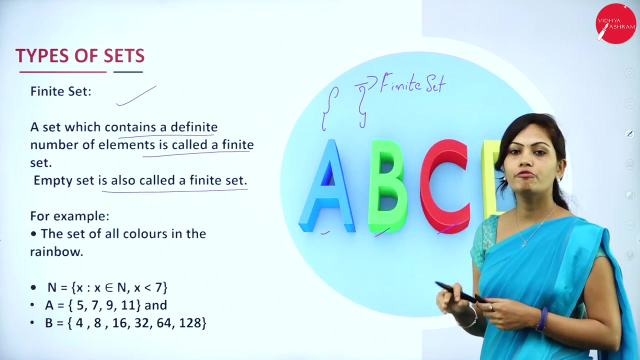 Empty set is also called a finite set. So empty set means there is no elements in a set. We can call it, as it is, a finite set also. So finite set means a set which contains definite number of elements. So if you are able to count the number of elements, we can call it as finite set. So finite set means a set which contains definite number of elements. So if you are able to count the number of elements, we can call it as finite set. So finite set means a set which contains definite number of elements. So if you are able to count the number of elements, we can call it as finite set. 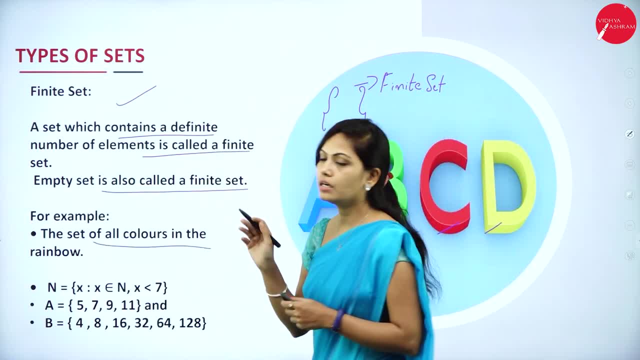 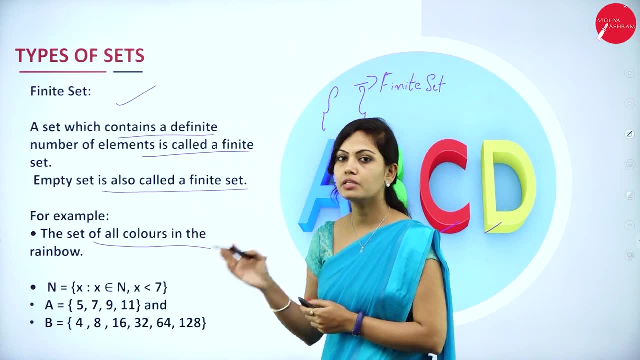 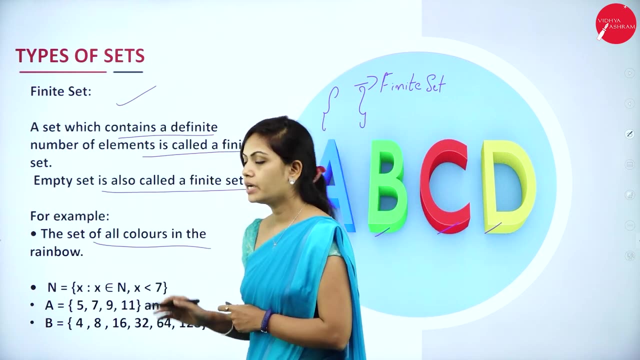 Example: the set of all colors in the rainbow. So here we are able to count the colors in the rainbow. So is it finite set? Yes, of course this is finite set example. So I can call: this is a finite set. And another example: 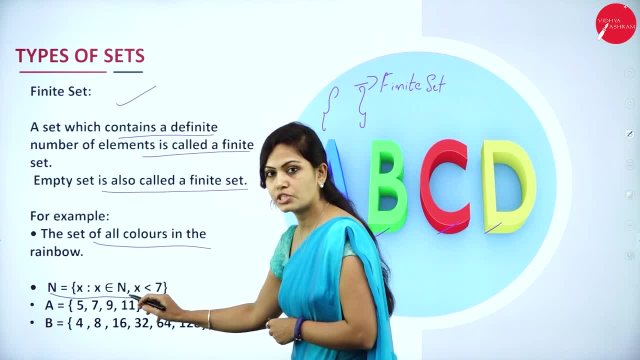 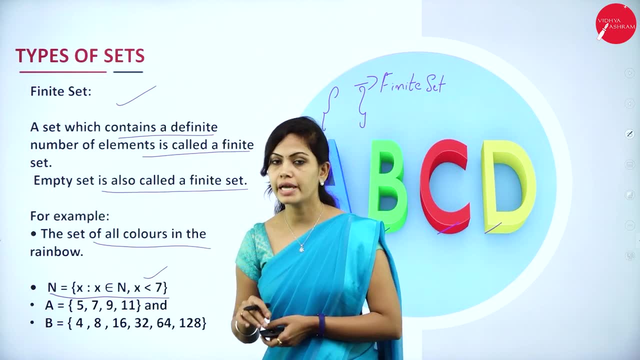 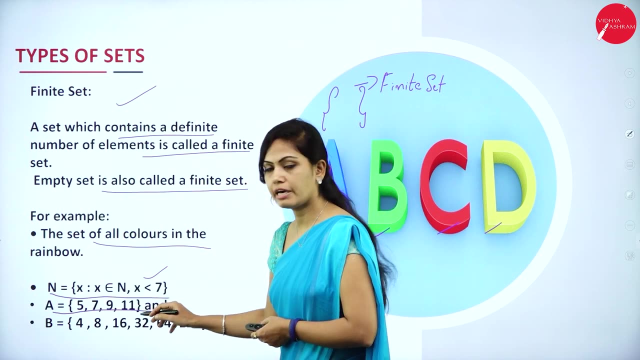 N is equal to X, such that X belongs to N. X is less than 7.. So X less than 7 means So we will get only 6 digits right And A is equal to. we have number of elements 5,, 7,, 9,, 11.. 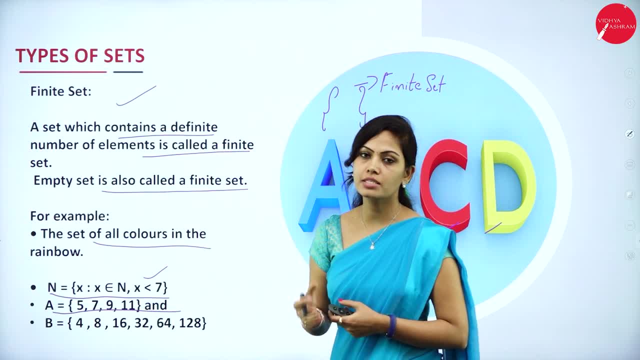 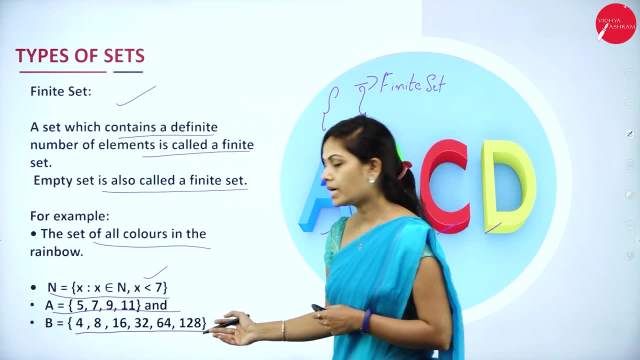 I am able to count this number of elements. So I can call it, as it is, a finite set, And B is equal to 4,, 8,, 16,, 32,, 64 and 128.. So easily I can count this number of elements. 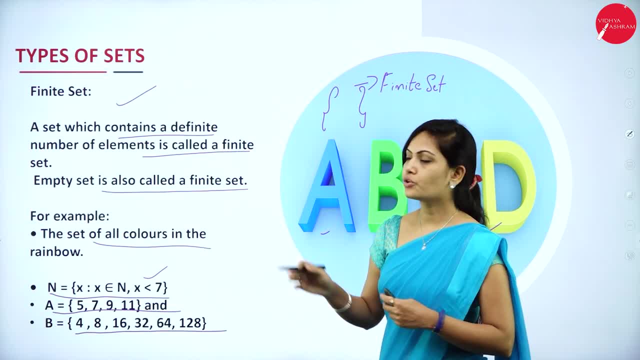 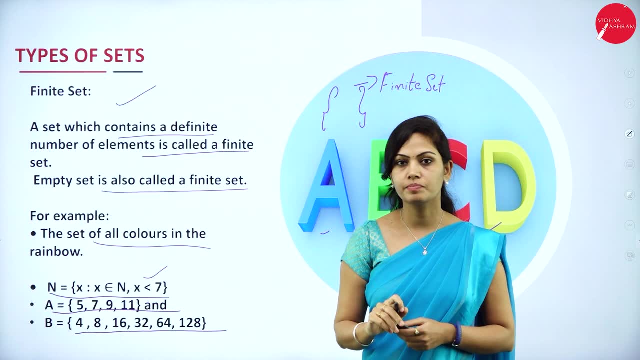 So I can call it as empty set. So empty set is a set which contains a definite number of elements. So empty set is a set which contains a definite number of elements. This is called as empty set. So null set or empty set is a finite set. 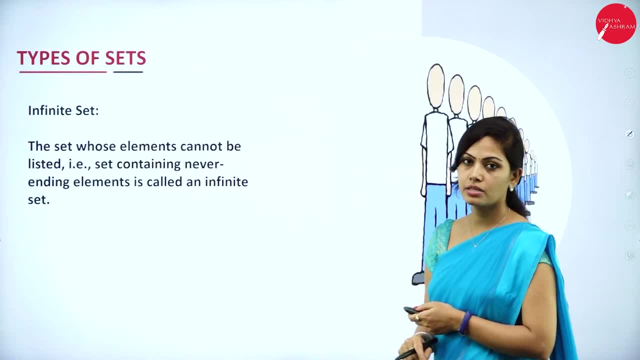 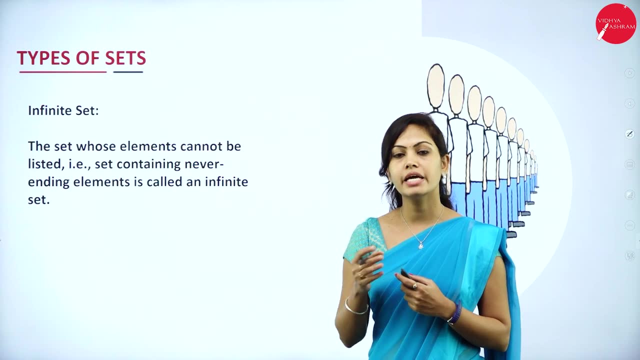 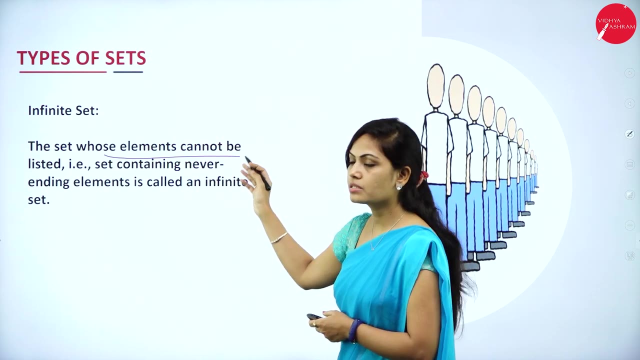 And the next type is infinite set. So what is infinite? So we are not able to count the number of elements. That is called as infinite set, The set whose elements cannot be listed, The set elements which cannot be listed, is called as infinite sets. 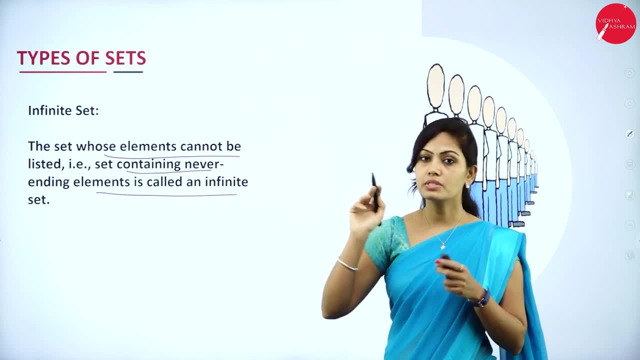 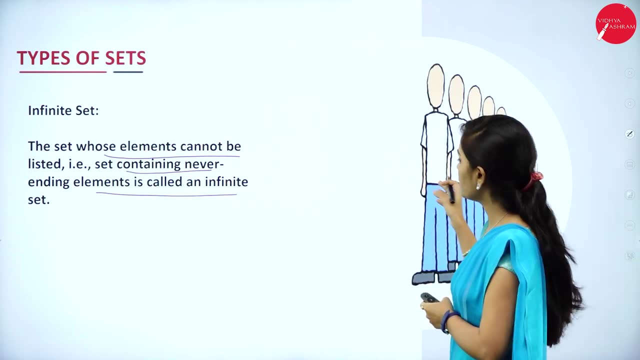 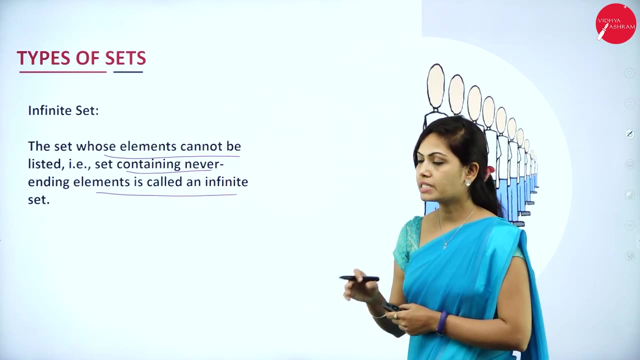 The set containing never ending elements. So set containing never ending elements is called as infinite sets. So here I am not able to count the number of elements in a set. We can call it as infinite sets. So infinite set means whose elements cannot be listed, or set containing never ending elements. 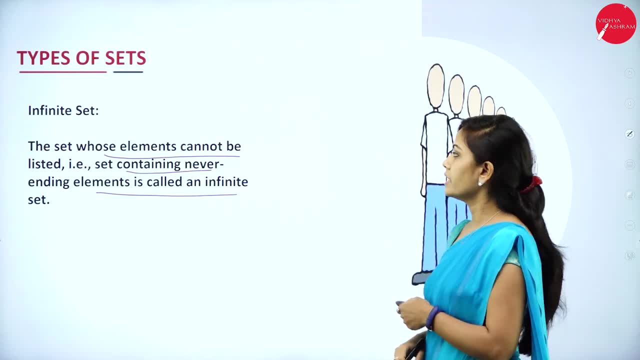 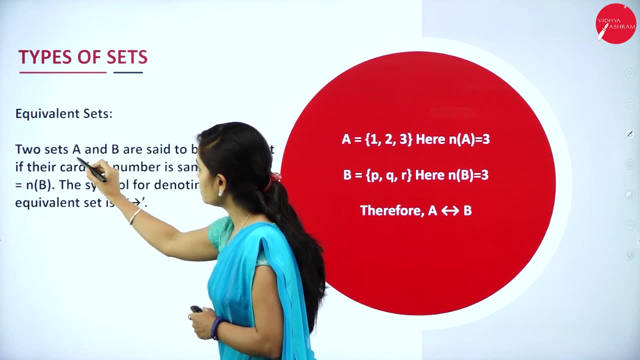 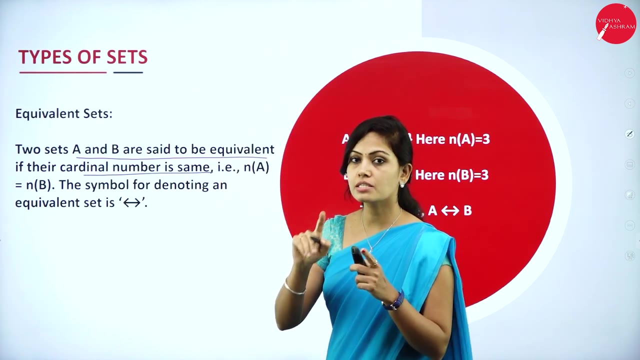 is called as infinite sets, And next is equivalent set. So what is this equivalent set? Two sets, A and B, are set to be equivalent if their cardinal number is same. Already I have discussed cardinal number. Example A is equal to 2,, 4 and 6.. 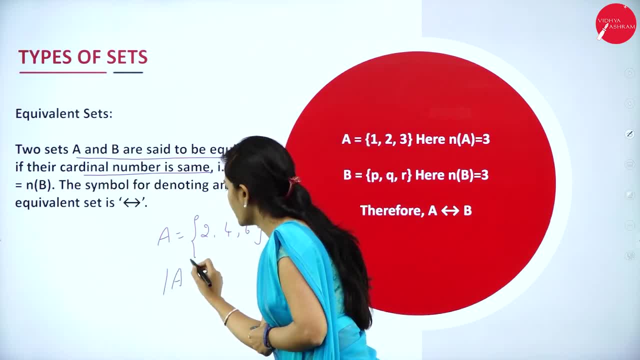 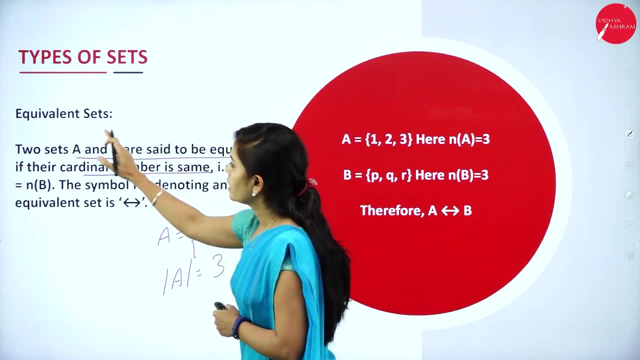 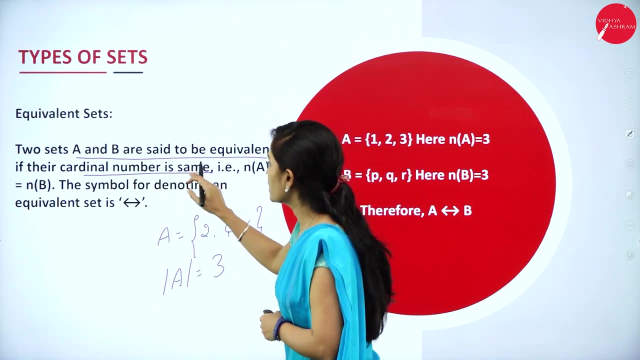 What is the cardinality of this number? So mod A is equal to 3.. We have three number of elements, So cardinality of this number is 3.. So here, equivalent set In equivalent set, two sets, A and B, are set to be equivalent if their cardinal number. 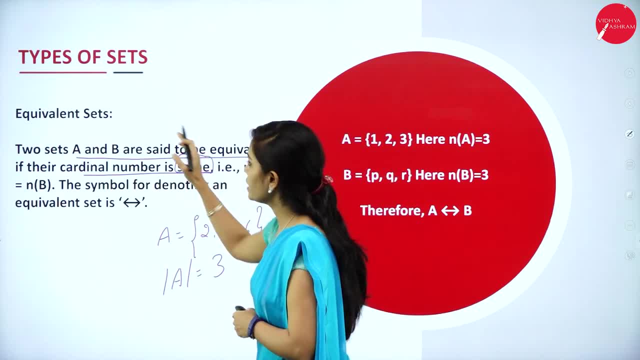 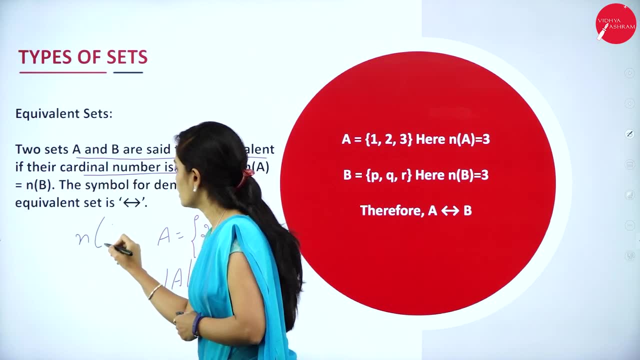 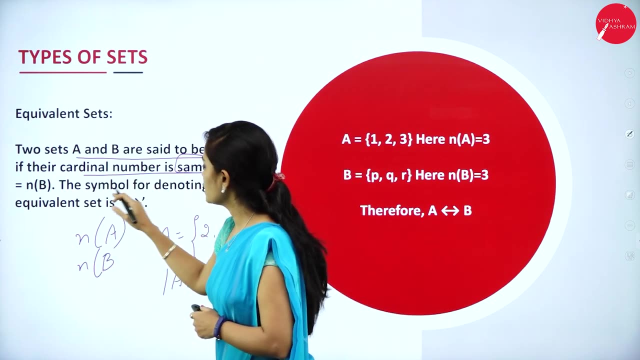 is same. If their cardinal number is same, means we can call it, as it is, an equivalent set, So we can represent it by N of A, N of B, etc. So this is equivalent set representation. The symbol for denoting an equivalent set is: 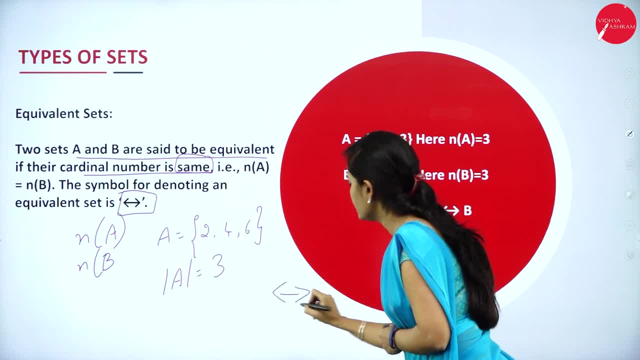 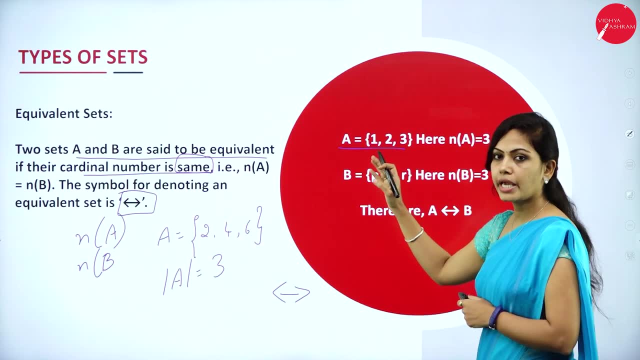 This is the symbol for representation, For representing equivalent set. Example: if A is equal to 1,, 2,, 3.. What is the cardinality of this set element A? So here I have three number of elements. So N of A is equal to 3.. 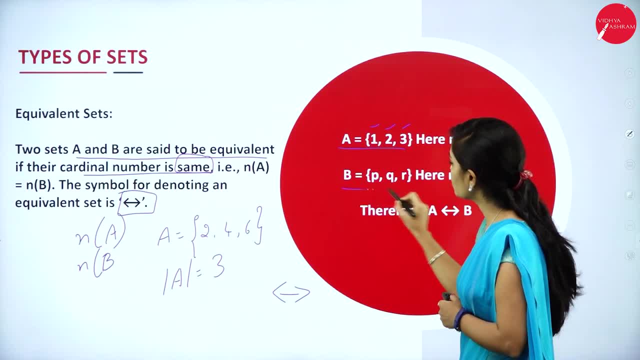 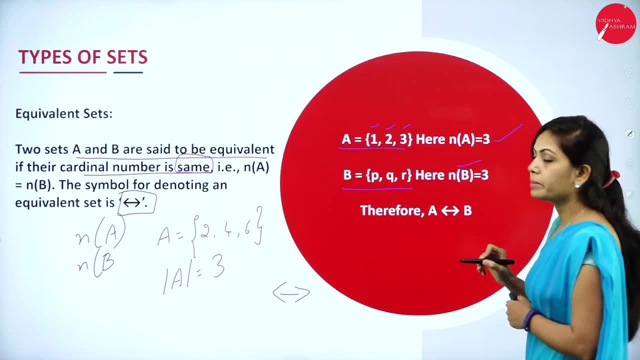 So this is an equivalent set representation and B is equal to PQR. We have three number of elements, So N of B is equal to 3.. You just compare this set elements of A and set elements of B. So cardinality of this set. 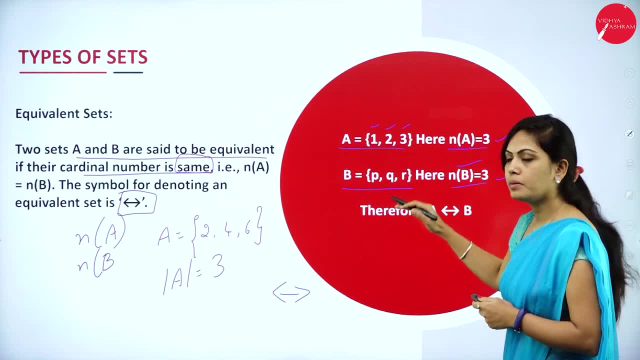 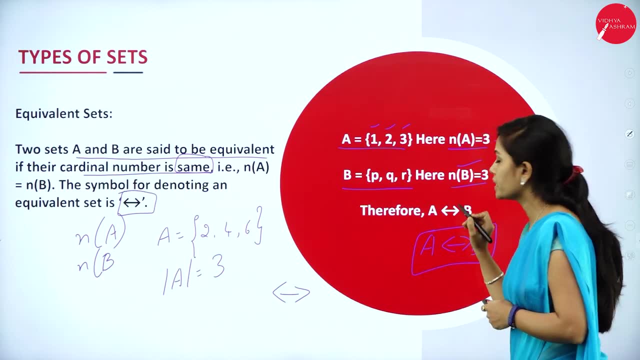 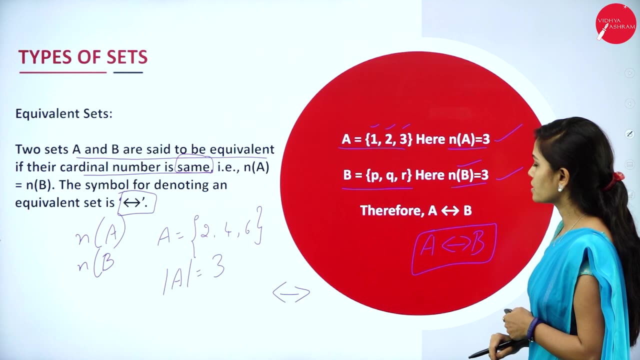 Cardinality is same in both set, A and B. Therefore A is equivalent to B. If the cardinal number is same in a set, we can call it as it is an equivalent set. And next we have equal sets. So what is this? equal sets and equivalent set. 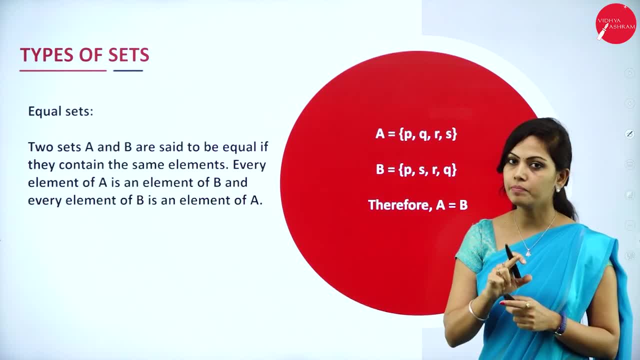 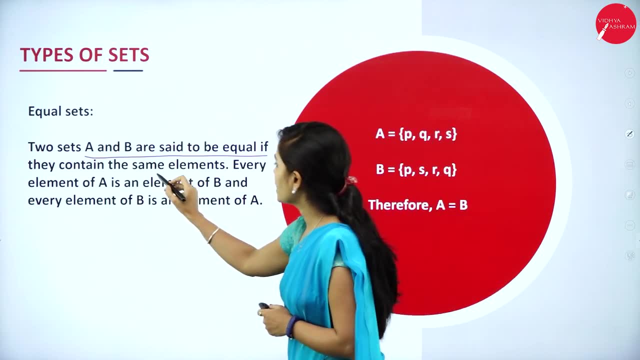 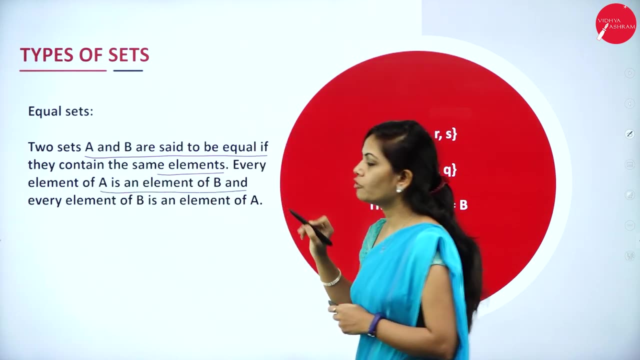 In equivalent set the cardinal number of sets is same, But in equal set Two sets, A and B, are set to be equal if they contain the same elements. If they contain the same elements, Every element of A is an element of B. Please understand the concept properly. 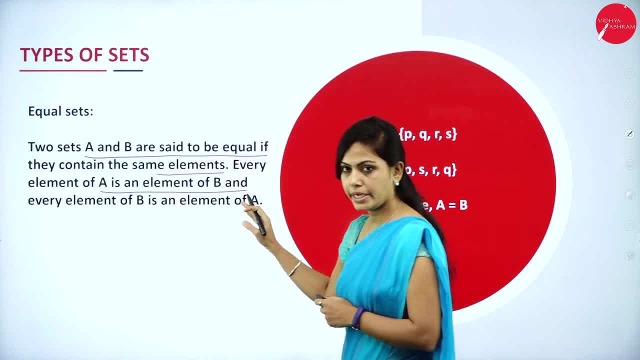 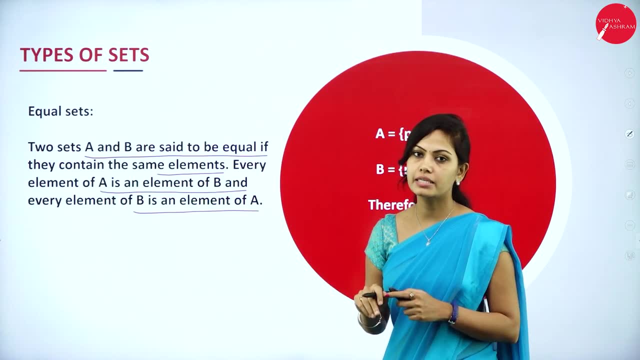 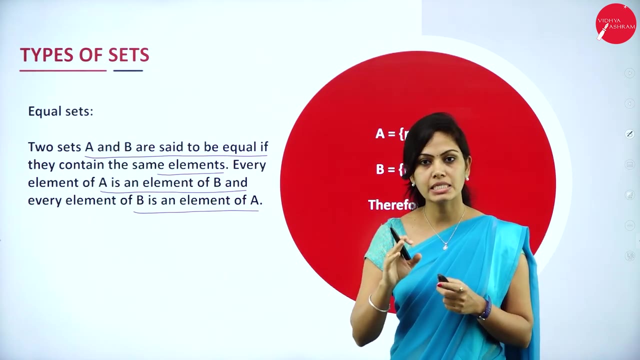 Every element of A is an element of B And every element of B is an element of A. We can call it as equal sets, But in equivalent sets All the cardinal numbers of A are equal sets, But in equivalent sets All the elements of set A and B or C should be same. 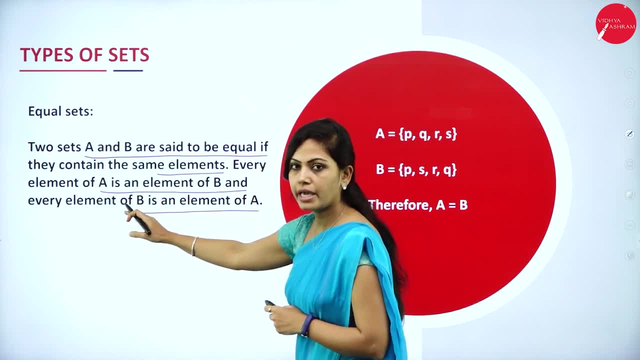 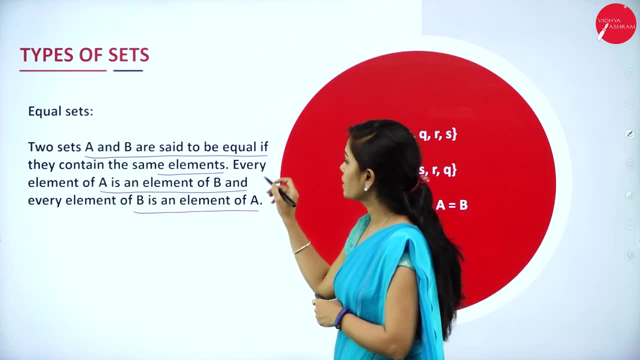 But in equal set, All the elements of set A is an element of B And all the elements of B is an set element of A. But in equal set, Every element of A is an element of B And every element of B is an element of A. 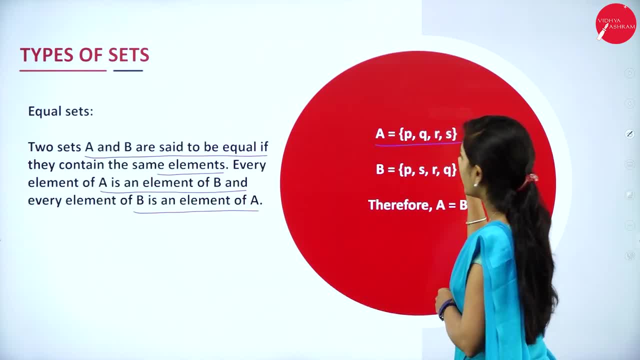 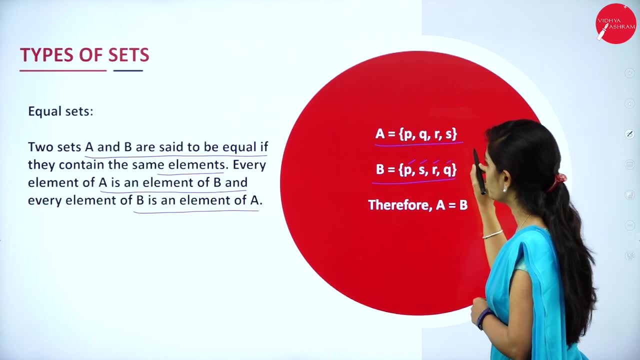 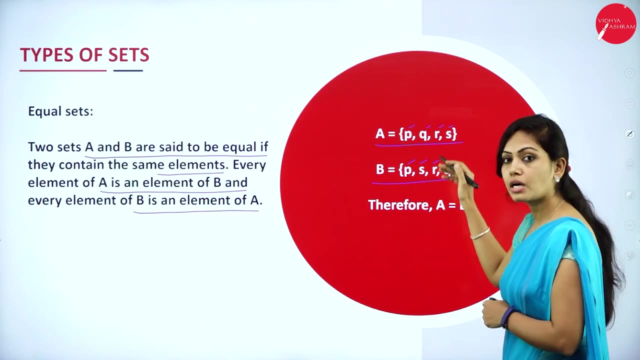 This is called as equal sets. Example A is equal to PQRS. We have four sets And in B We have PSA, SRQ. You just observe these two elements, PQRS and PSRQ. both are same but not in order. 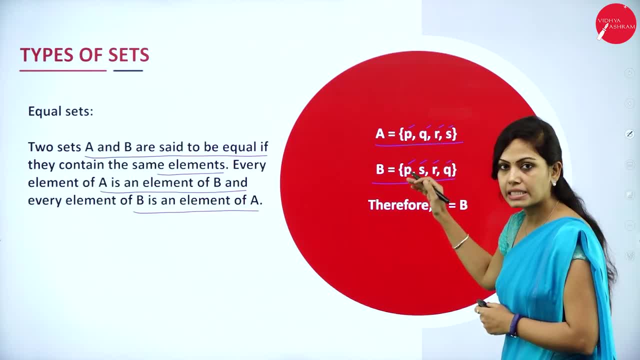 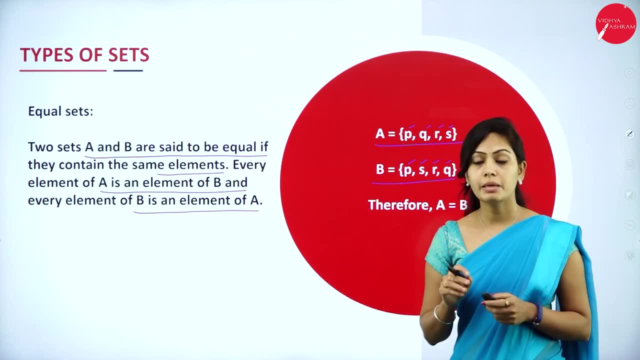 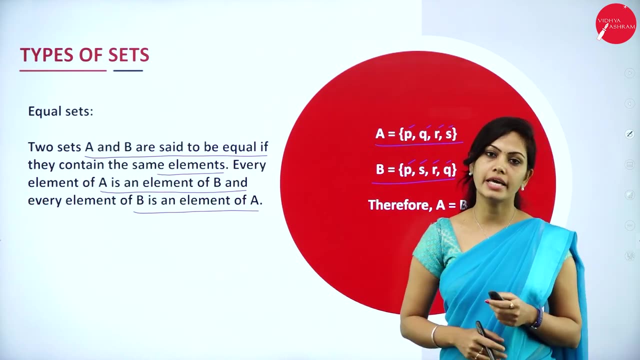 So in these two sets both the elements are same but not in proper order. So we can call it as this: equal sets. Keep in mind, in sets all the elements or objects are not in proper order. Then also we can call it as a set. 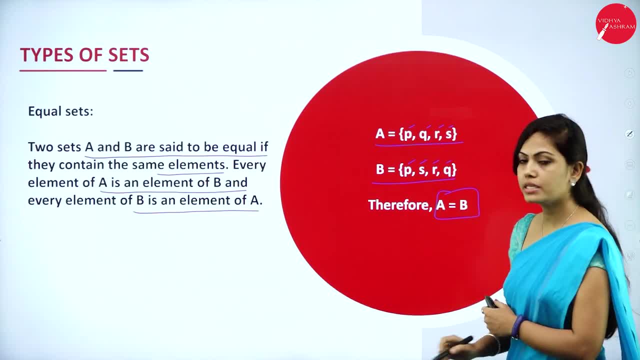 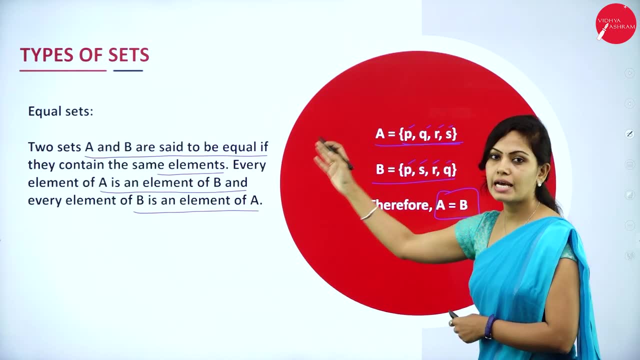 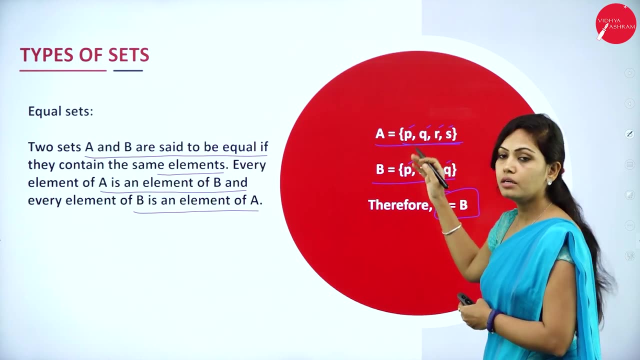 So this is the representation of equal set. A is equal to B Because every element of A is an element of B, we can call it, as is, an equal sets. See the difference of equivalent and equal set. So here both the elements are same in equal sets. 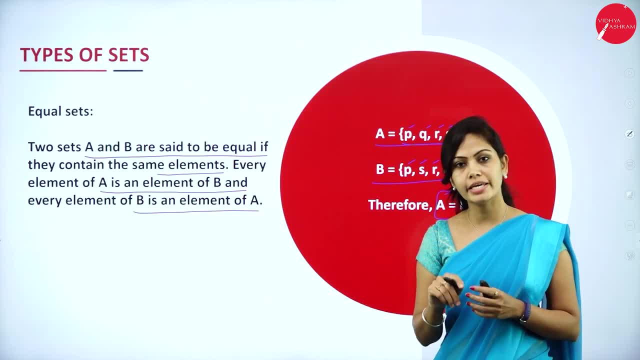 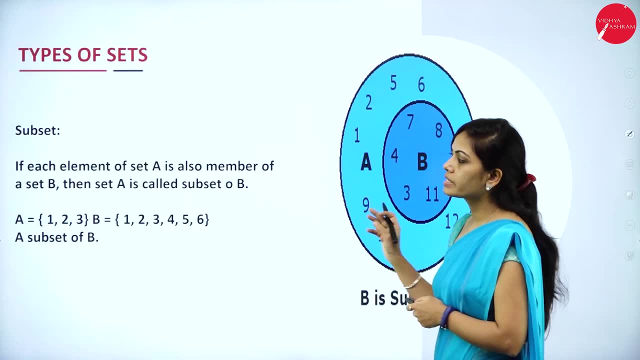 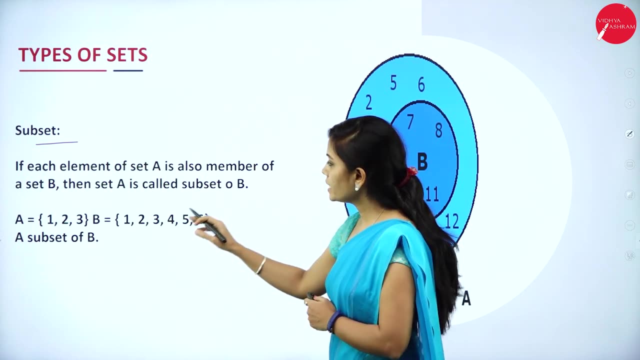 But in equivalent set. all the cardinality should be same in equivalent set. So this is your equal set and equivalent set. And next type is subset. Very important question for two marks: What is subset If each element of A is also member of a set B? 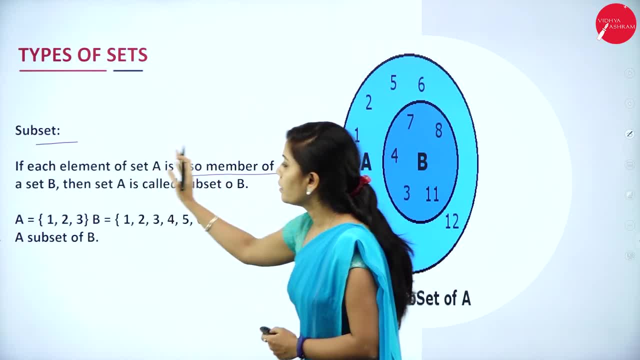 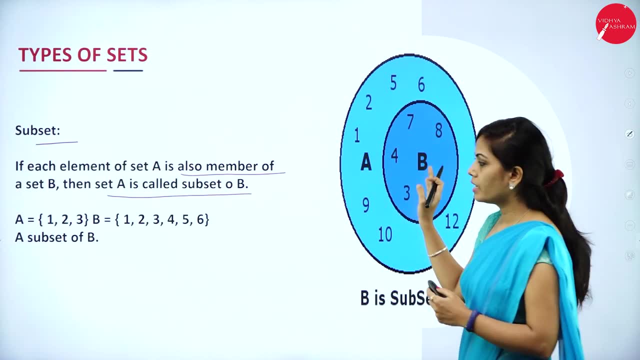 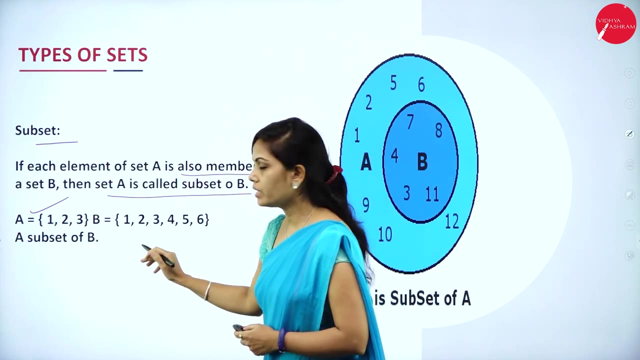 If each element of set A is also member of set B, Then set A is called subset of B. Example: Here I have set element 1,, 2, 3, and in set B I have 1,, 2,, 3,, 4,, 5, 6.. 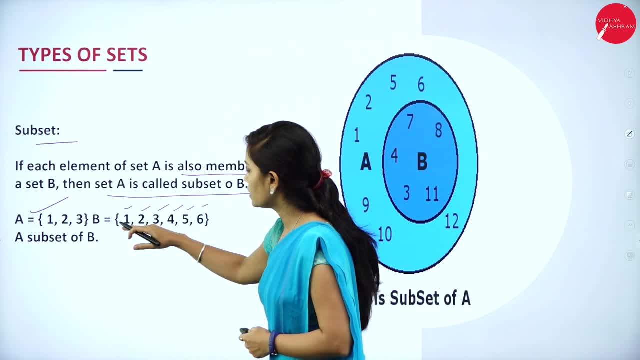 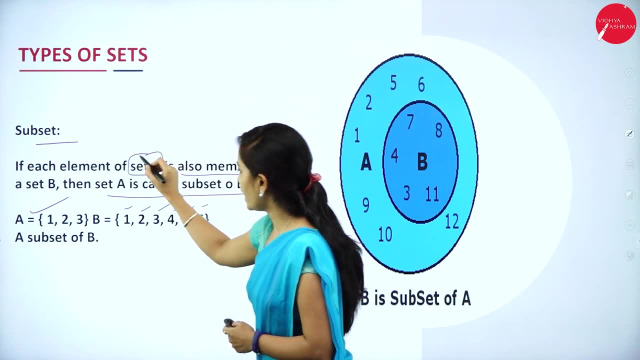 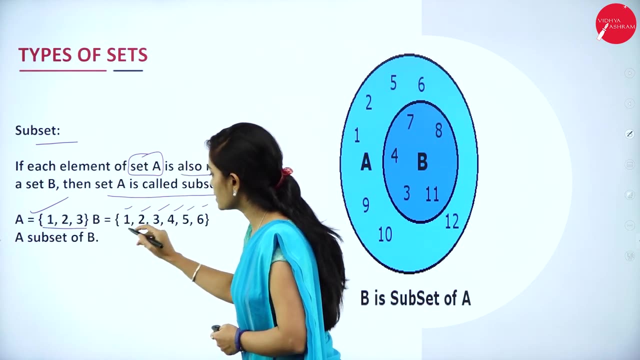 Here the number of element is 3, but in B the number of element is 6.. Understand the concept If each element of set A is also a member of set B. So in set A I have 1,, 2, 3 and also in set B I have same element called 1,, 2, 3.. 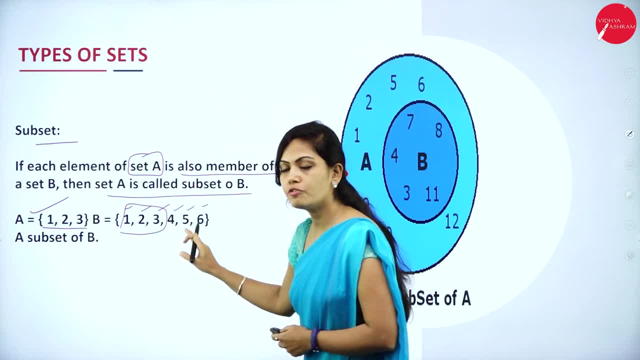 So I can call it as A is equal to B. So in set A I have 1,, 2, 3, and also in set B I have same element called 1, 2, 3.. So I can call it as A is a subset of B. 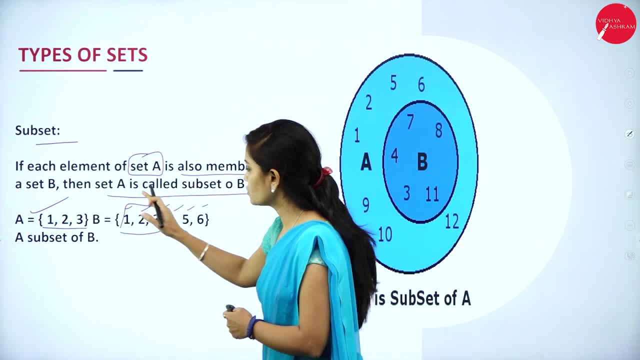 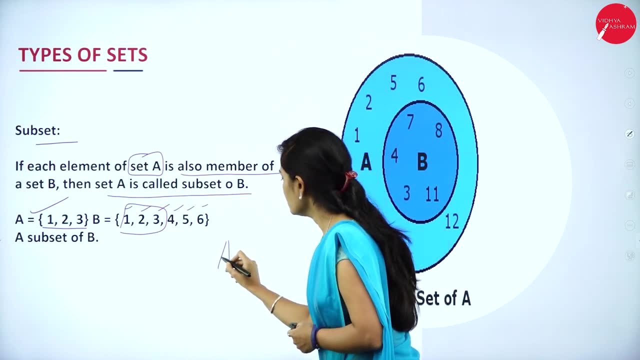 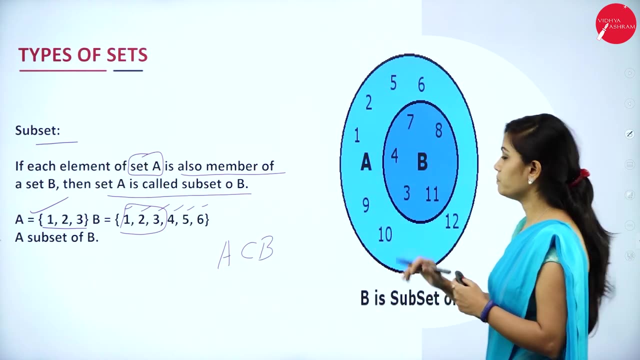 Because each element of set A is also a member of element of set B. I can call it as: A is a subset of B, So you can represent it by this symbol: A is an element of B. So here you can observe this: B is a subset of A. 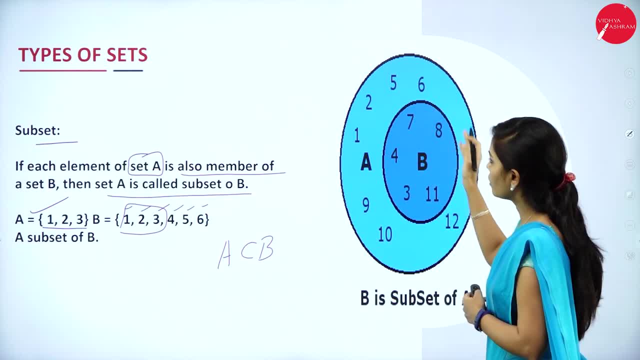 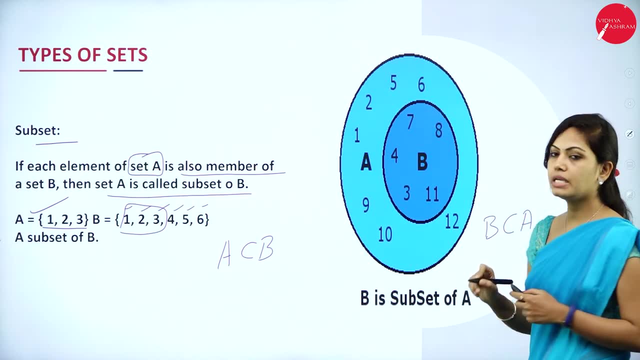 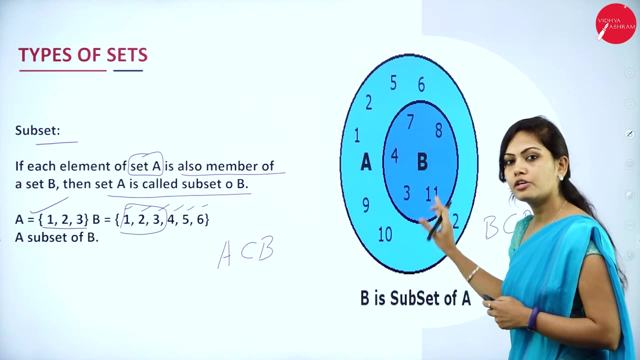 Because every element of B is also an element of A. So I can call B is a subset of A. B is a subset of A Because every element of B is also an element of A. I can call it as subset, So this is called as subset. 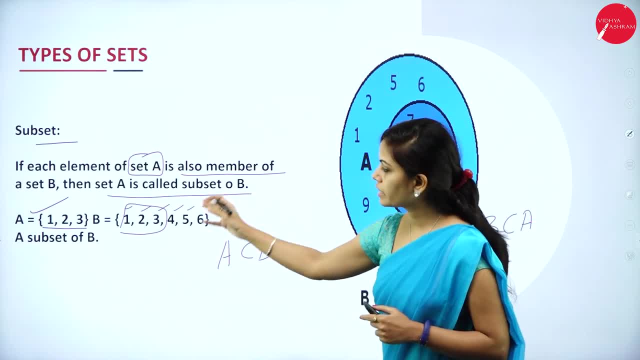 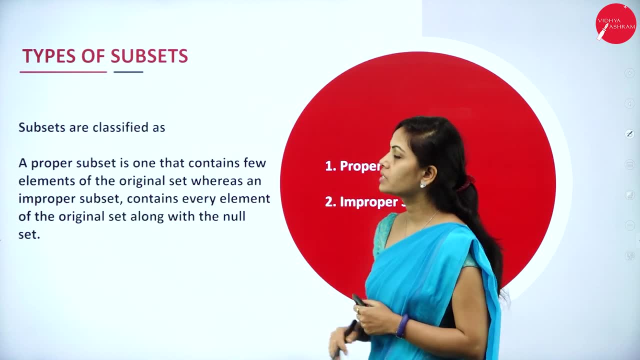 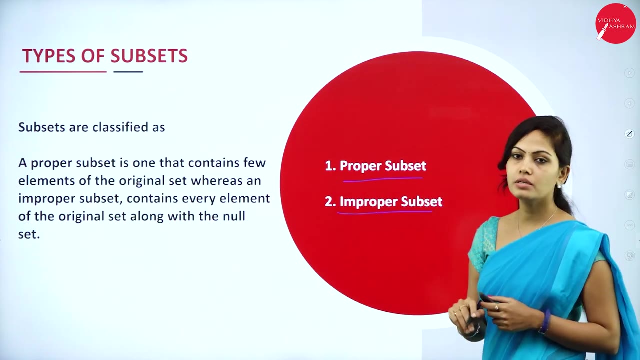 Very important question for 2 marks: What is subset? Give an example So you can write any example for subset. So next topic is types of subsets. So in subsets We have 2 types, that is, proper subset and improper subset. Proper subset and improper subset. 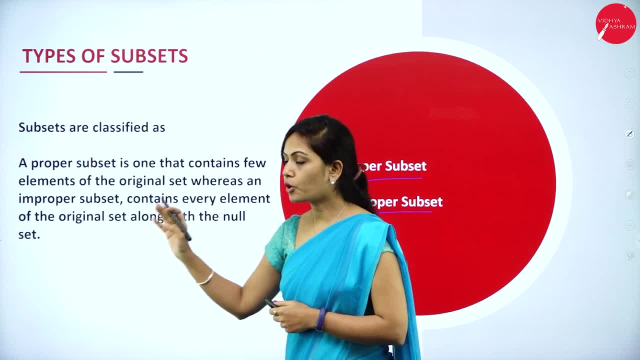 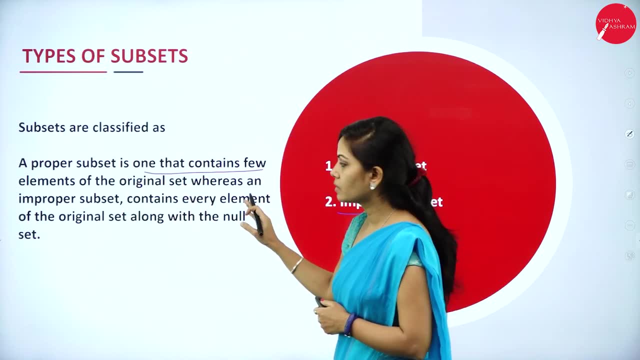 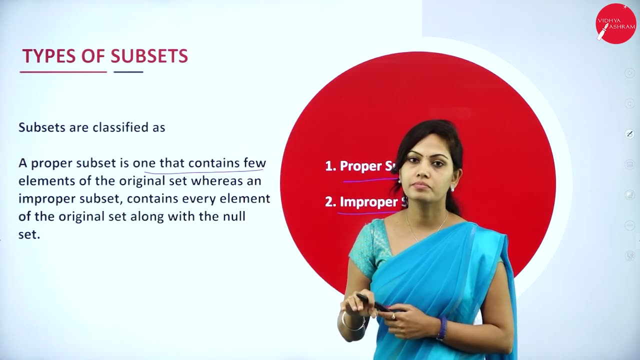 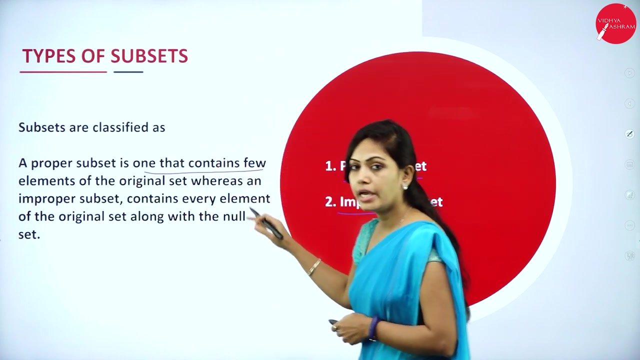 So what is this proper subset? So a proper subset is one that contains few elements of the virginal set, whereas improper set contains every element of the virginal set, along with the null set. Already I have discussed the subset. So in subset we have 2 categories, that is, proper set and improper set. 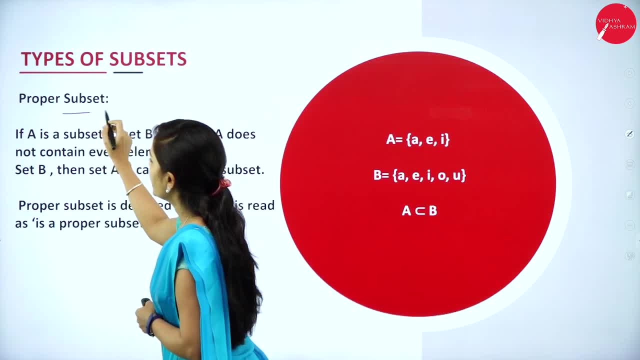 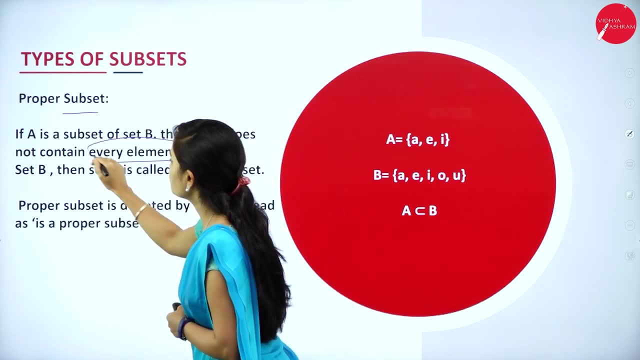 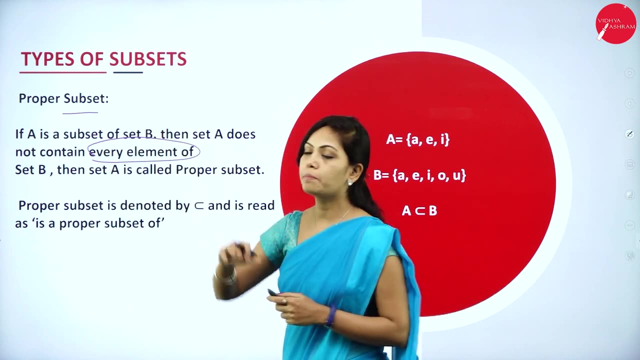 So let us understand with an example. Proper set: If A is a subset of B, then set A does not contain every element of set B. If A is does not contain every element of set B, I can call it as this: a proper subset. 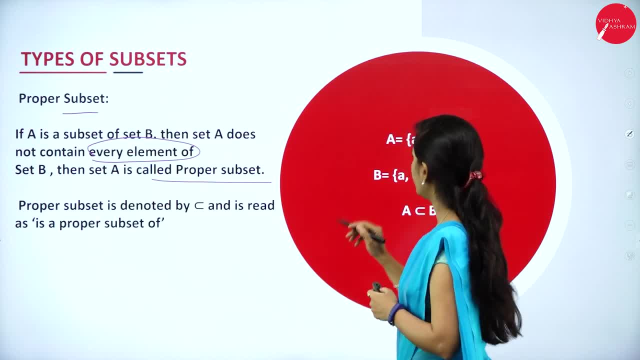 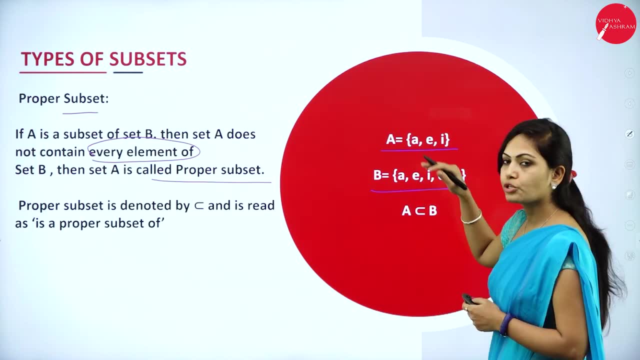 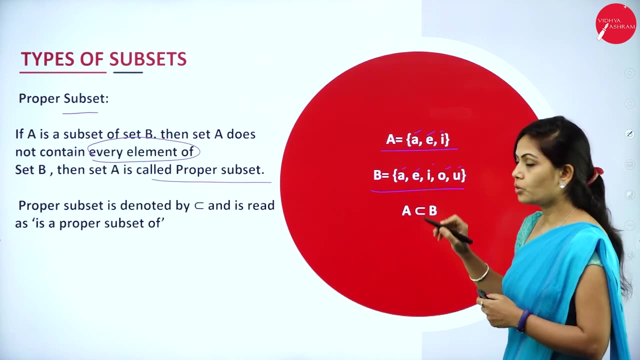 Then set A is called proper subset. Example: If A is equal to A, E, I and B is equal to A, E, I, O, U. So here in set A I have 3 elements, in set B I have 5 elements. So what is the definition? 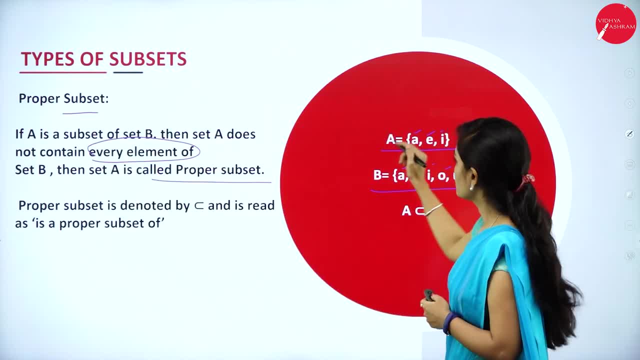 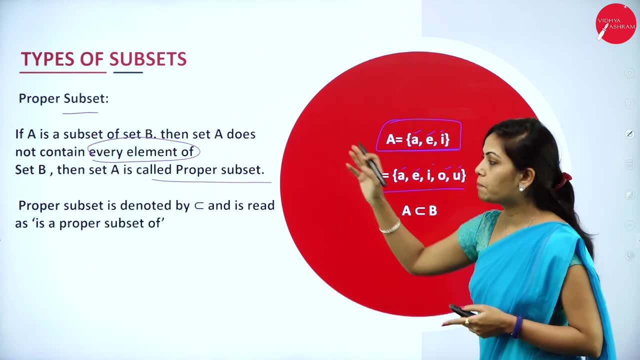 Set A does not contain every element of set B. The set A does not contain every element of set B, then I can call it as it is, a proper subset. So the set A does not contain every element of set B, then I can call it as it is a proper. 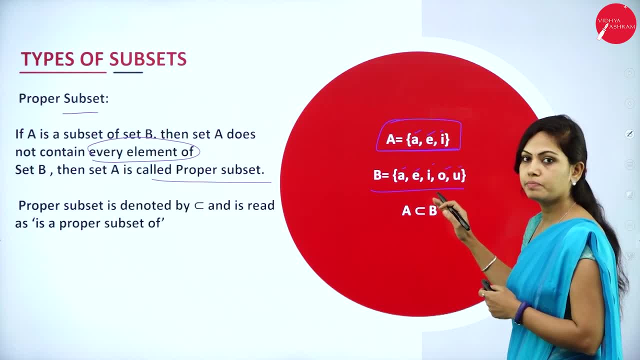 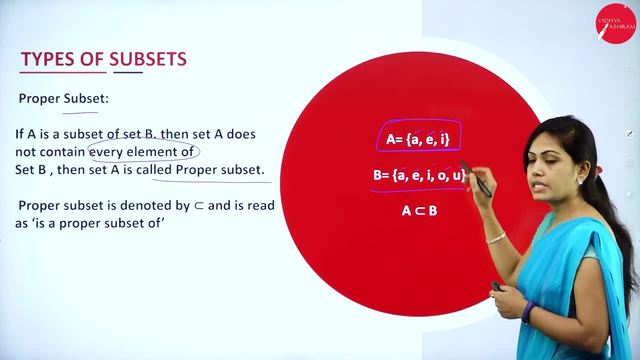 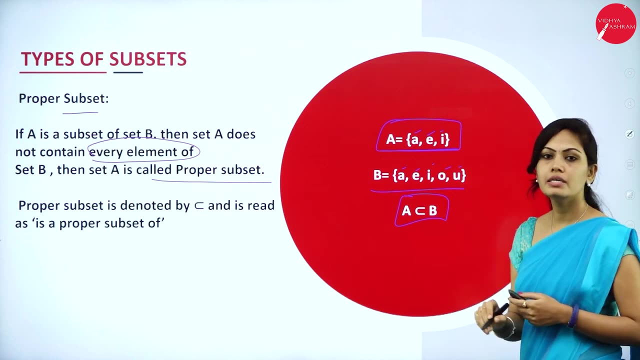 subset. The set B does not contain every element of set B, So here I have only A E I, but in set B I have A, E, I O U. Set A does not contain every element of set B. therefore I can call it as proper subset. 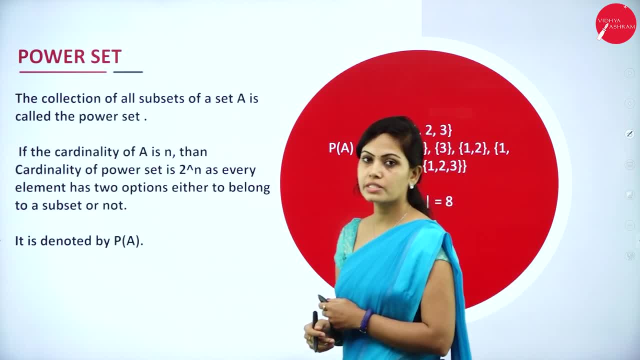 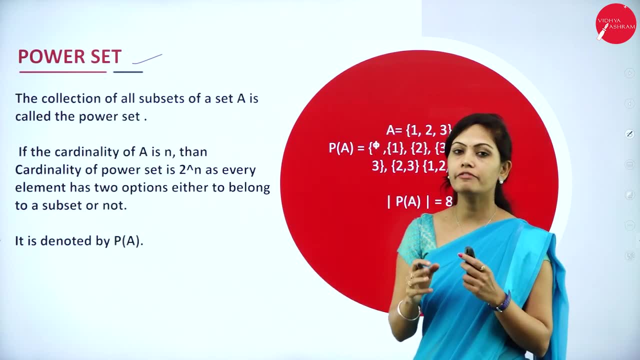 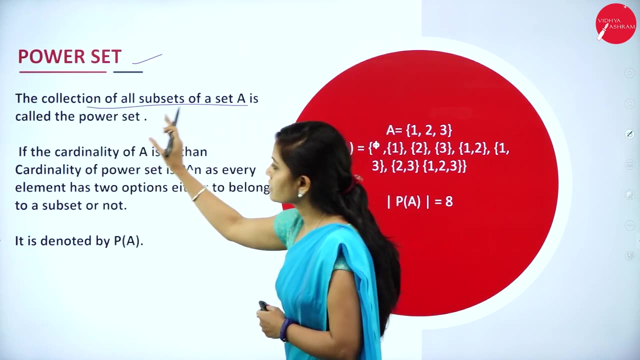 And next important concept is power set. Very important concept: power set. You can expect this question for 2 marks. What is power set And give an example. So what is power set? The collection of all subsets of a set A is called the power set. 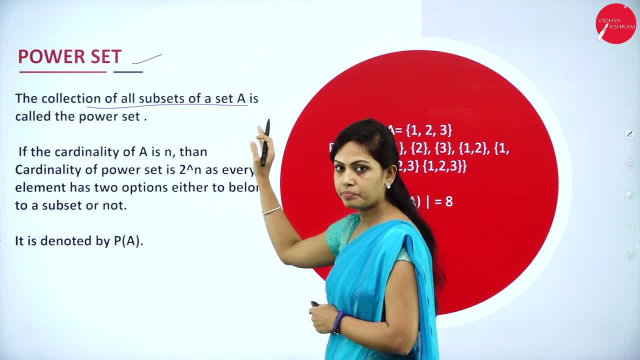 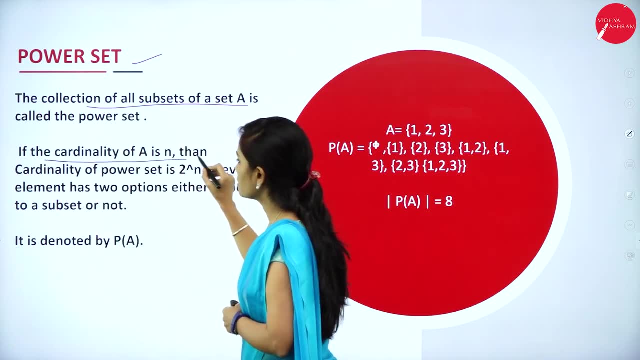 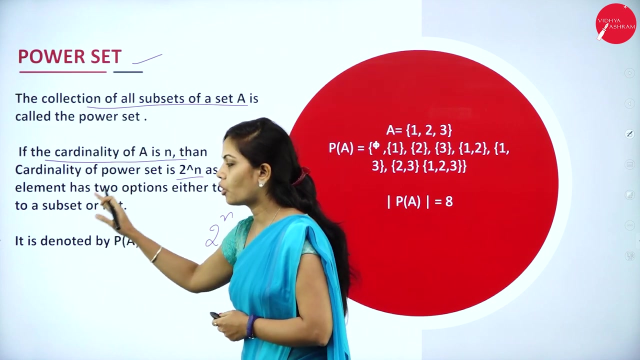 The collection of all subsets of a set A is called as power set. If the cardinality of a set A is n and cardinality power set is represented by 2 power n, as every element has 2 options: Either to belong to a set or not. 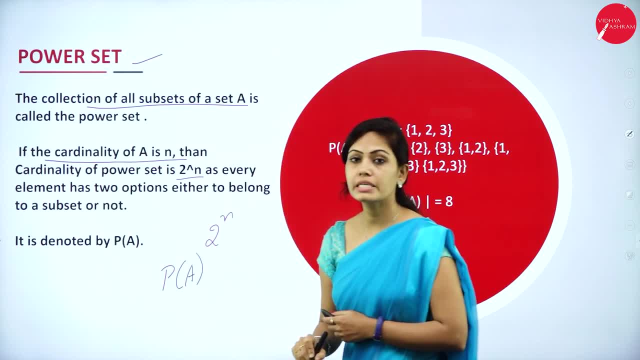 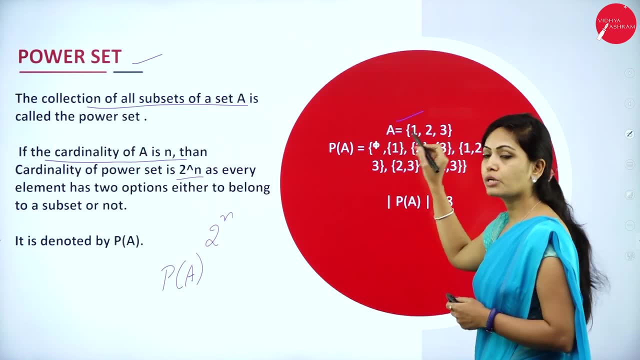 So it is denoted by P of A. So power set is denoted by P of A Example. so here I have set A. A is equal to 1,, 2, 3.. How to write it in a power set. 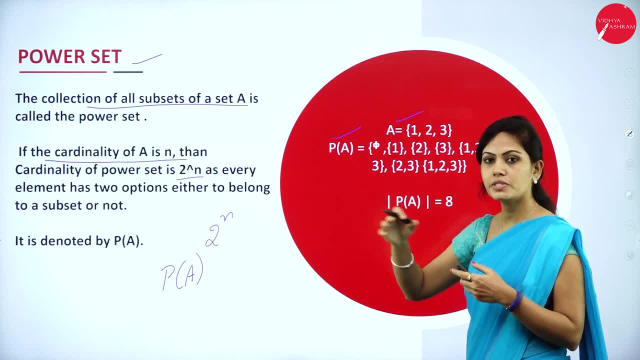 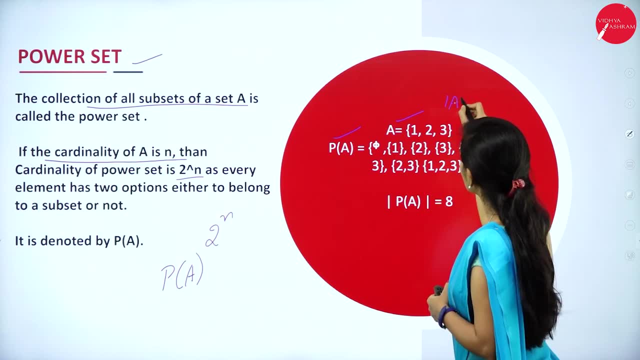 So it is represented by P of A, P of B, P of C, etc. So A is equal to 1,, 2,, 3.. Cardinality is so mod A is equal to what 3.. So cardinality of this set is 3.. 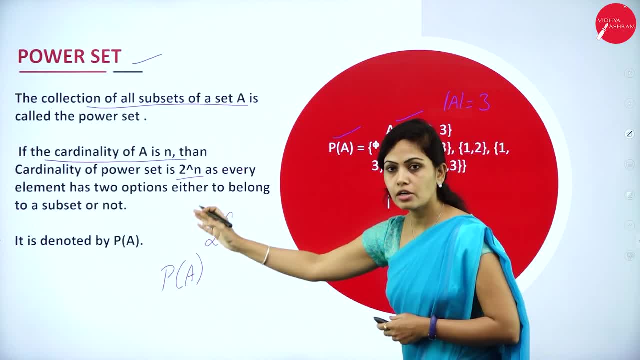 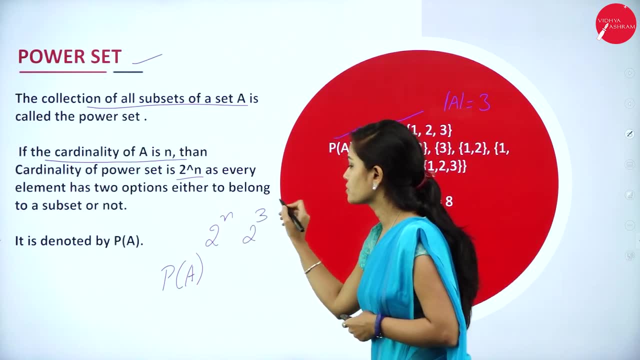 I have 3 number of elements. So what is the cardinality of a power set? So it is represented by 2 power n. So n is equal to 3.. So 2 power 3 is equal to. you will get 8 set elements. 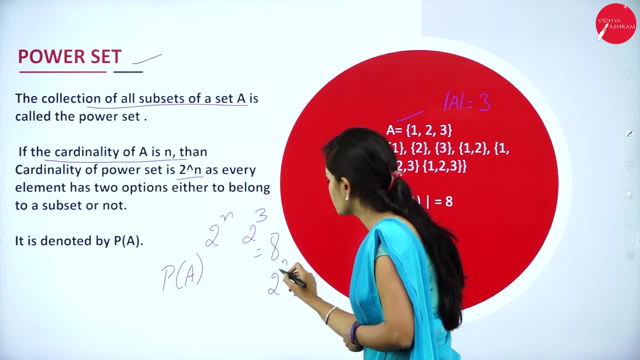 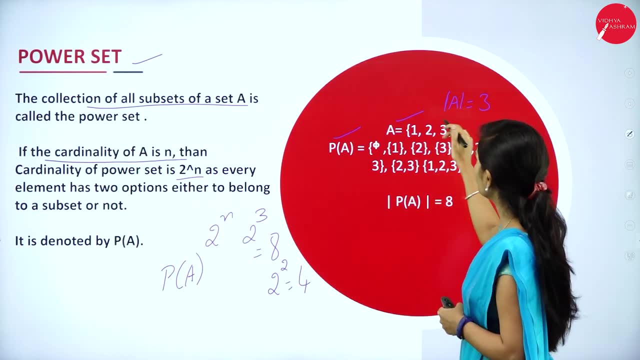 So if your cardinality is 2, so you will get 2. power 2 is equal to 4. number of elements. So, For example, so you have cardinality is equal to 3. So you will get 8. number of sets: 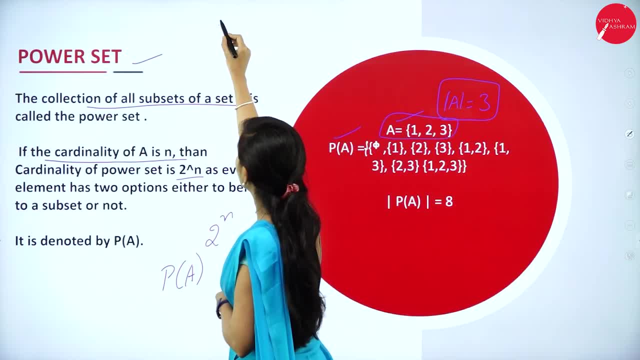 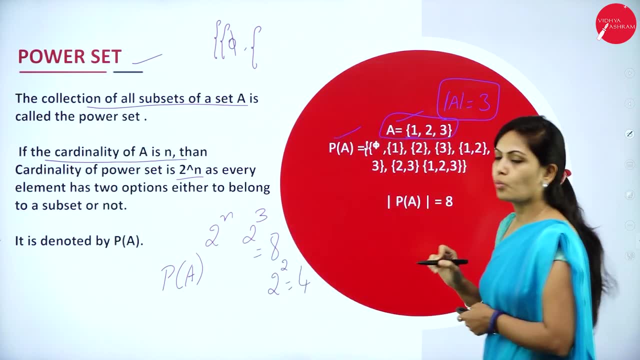 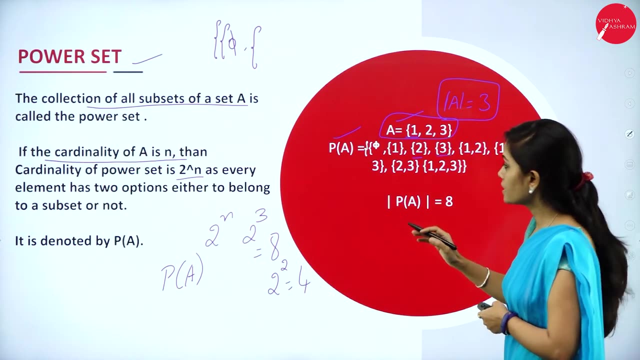 So how to write this power set? So you have to start with null set 5 comma. the first element is 1 and the second element is 2 and the third element is 3.. Starts with null value: open double flower bracket and null value comma: power 3.. 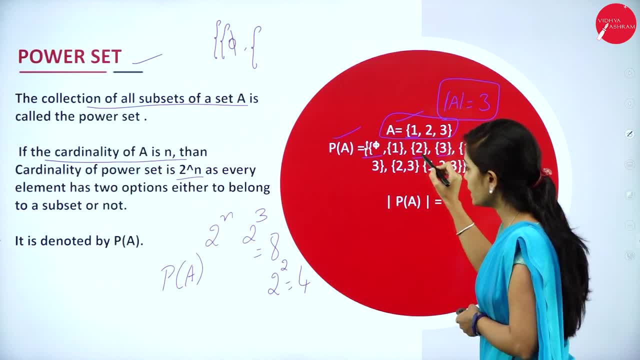 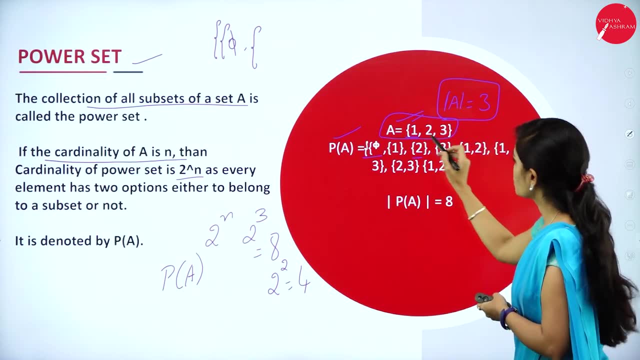 So you have, cardinality is equal to 3.. So you will get 8 number of sets, First element, second element and third element, And compare this first element with second element and third element, So 1 comma 2, 1 comma 2, 1 comma 3.. 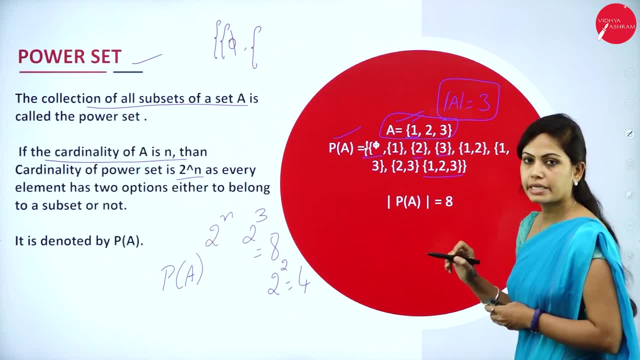 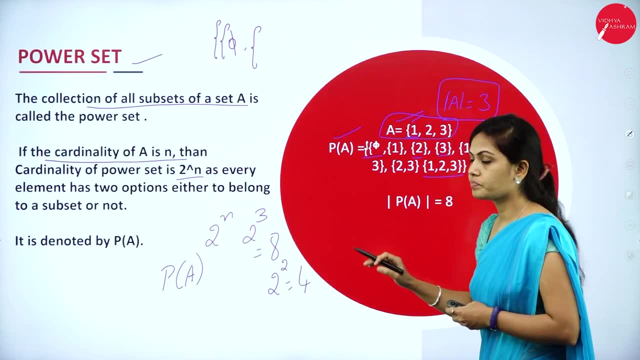 So totally, you will get 8 possible set elements: 1, 2, 3,, 4,, 5,, 6,, 7,, 8.. So 2 power 3 is equal to 8.. So I will give one more example. 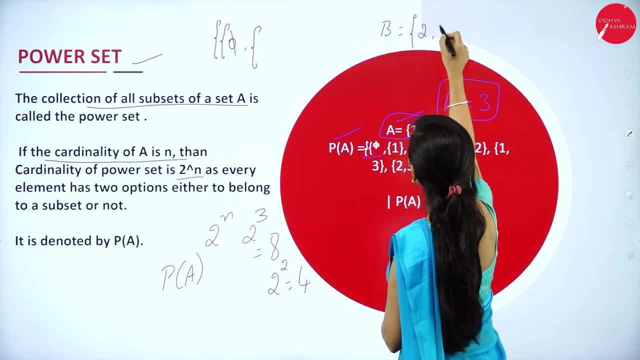 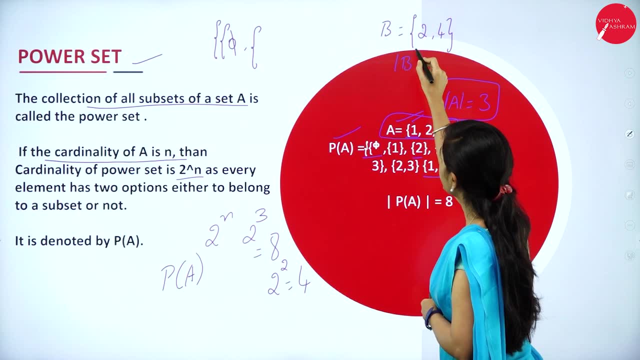 If set B is equal to 2 comma 3. So you have 2 power. 3 is equal to 8.. So I will give one more example. Here I have only 2 set elements, 2 comma 4.. So what is the cardinality? 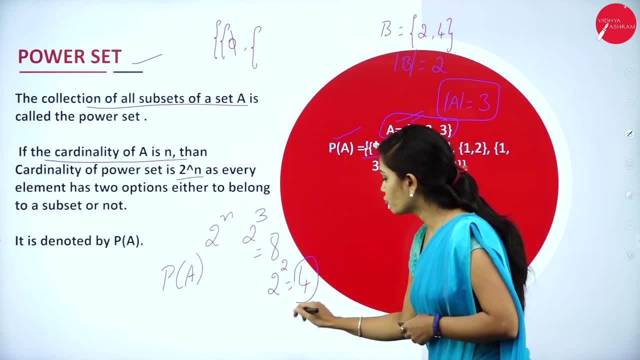 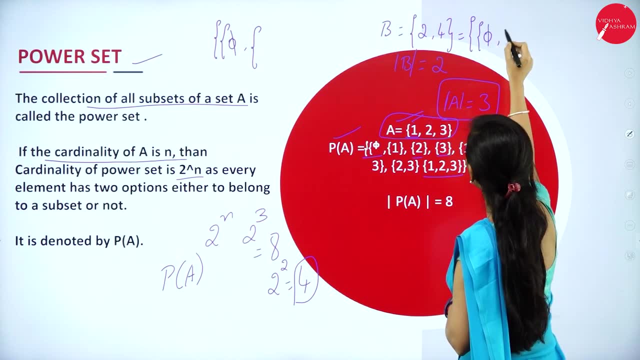 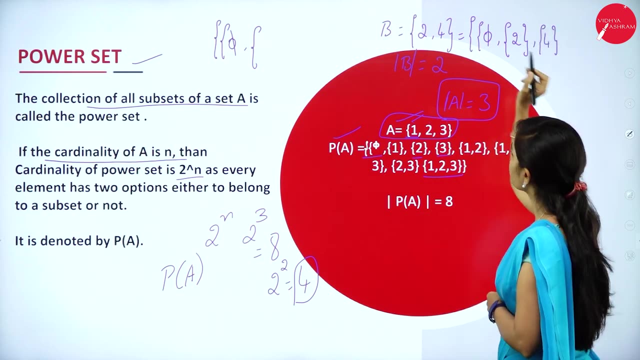 Mod B is equal to 2.. So 2 power 2 means you will get 4 number of elements. So you have to start with the 5. that is null set comma. first element is 2 and second element is 4.. And compare this first element with second element, that is 4.. 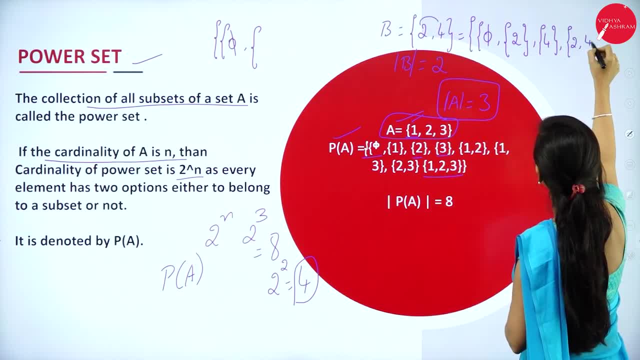 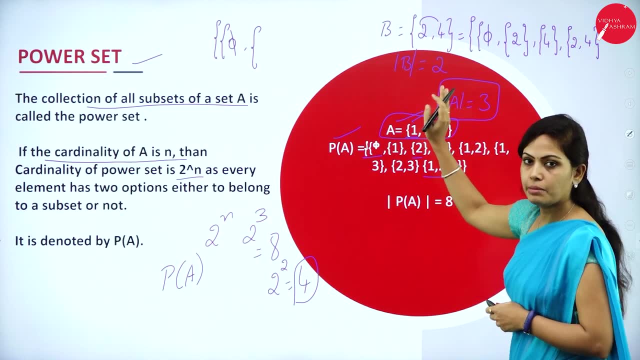 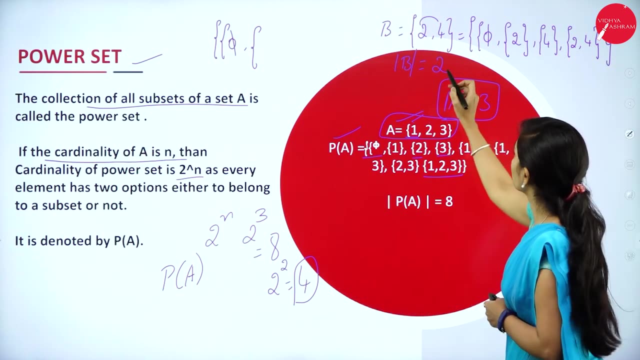 So you will get 4.. That is 2 comma 4.. Is there any other possibilities to compare with the third element? No, I have only 2 elements, So 1,, 2,, 3, 4.. So I have completed with the 4 number of elements. 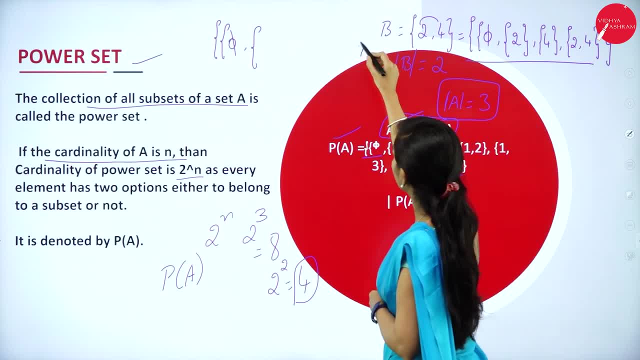 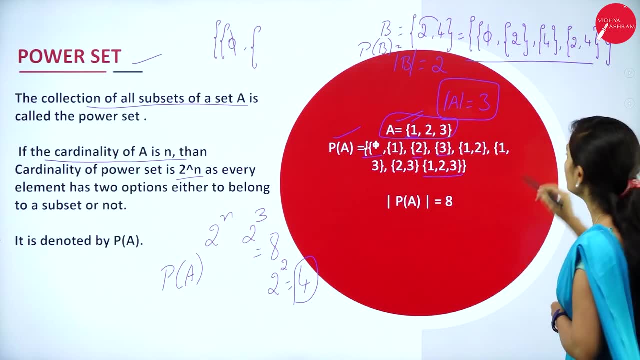 So this is your power set. So P of B is equal to 5,, 2,, 4 and 2 comma 4.. So you have to closed with double flower branch. So this is your power set. So P of B is equal to 5,, 2,, 4 and 2 comma 4.. So you have to closed with double flower branch.